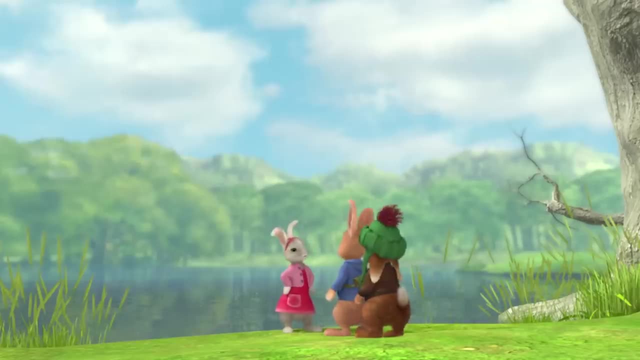 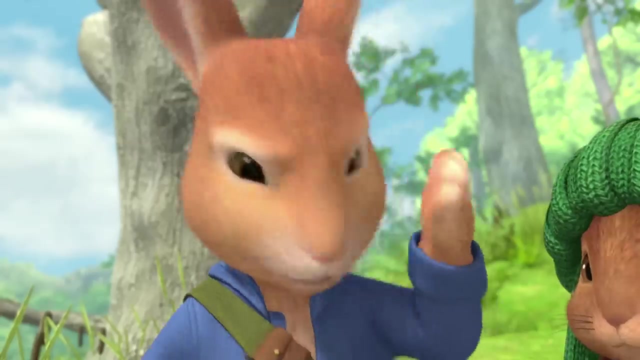 But I've got to get over there. What we need is a boat. Yes, We can build one. The plans are in my dad's journal. Oh, Oh. This is exactly why We need to get it back. Sigh. 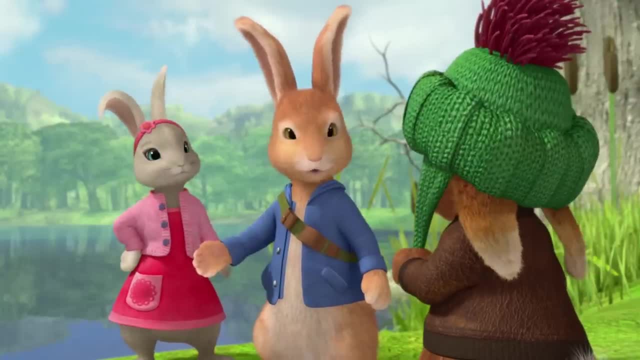 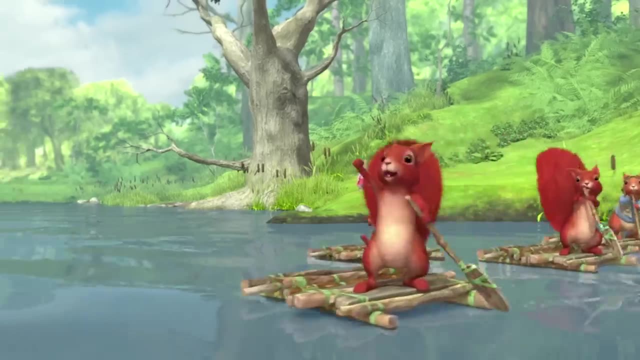 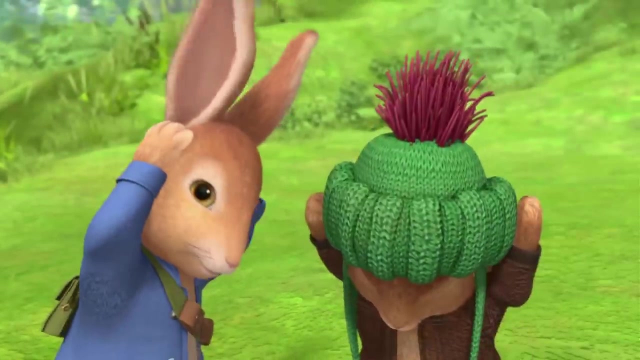 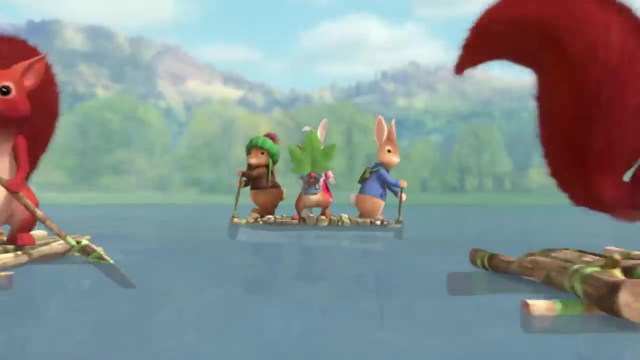 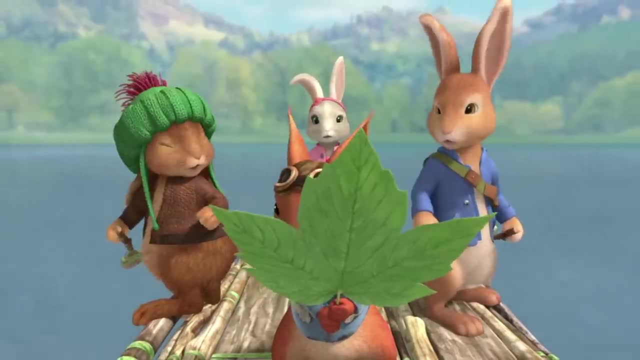 Ha-ha-ha, Ha-ha-ha, Ha-ha-ha, Ha-ha-ha, Ha-ha-ha. Thanks for the lift. Nutkin, I'm not Nutkin. Huh, Er, you're not. 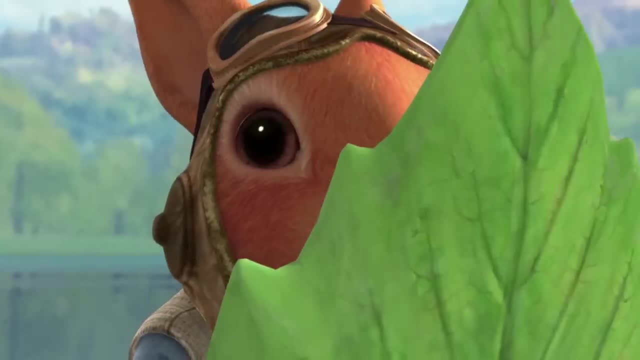 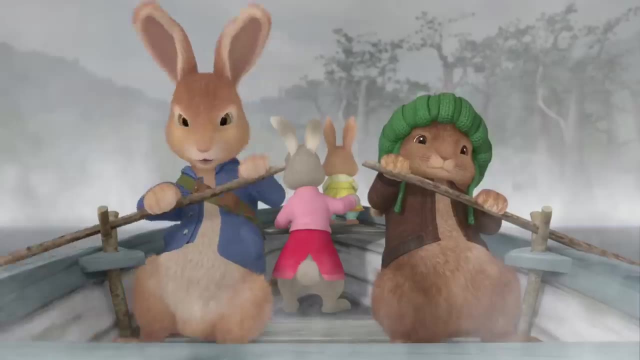 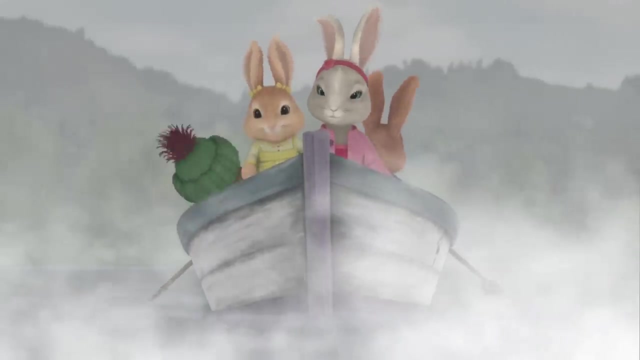 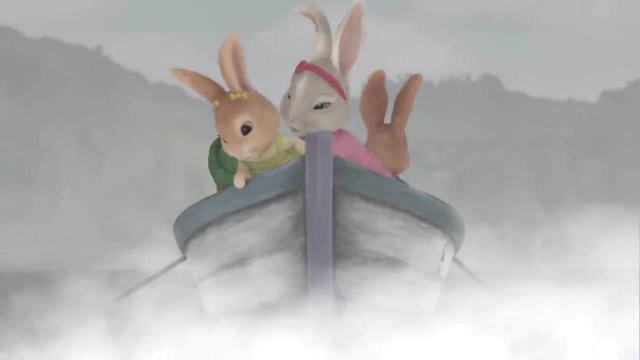 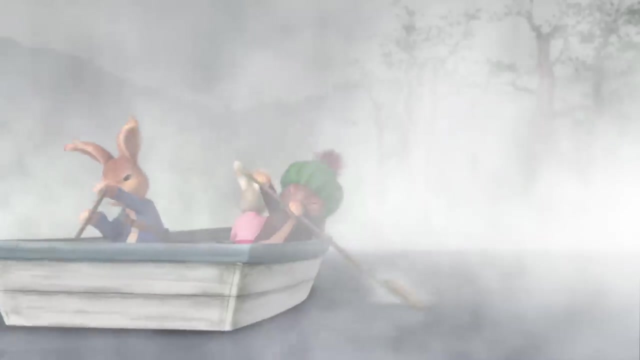 I'm not even a squirrel, And neither are my friends. You're all right, Lily. It is too far to swim, It's too far to row. Don't worry, I think we're almost there. How do you know? Because Rocky Island is always surrounded by mist. 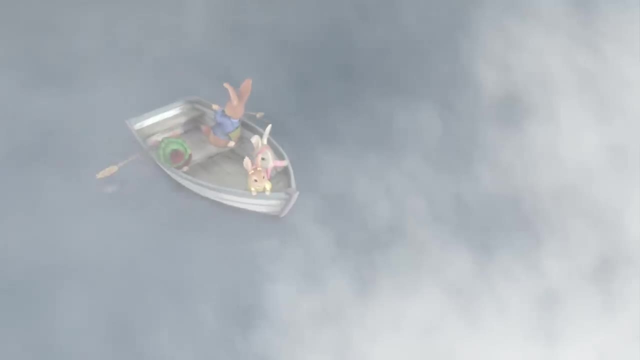 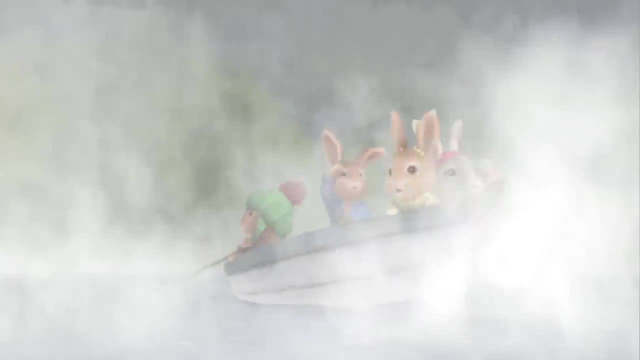 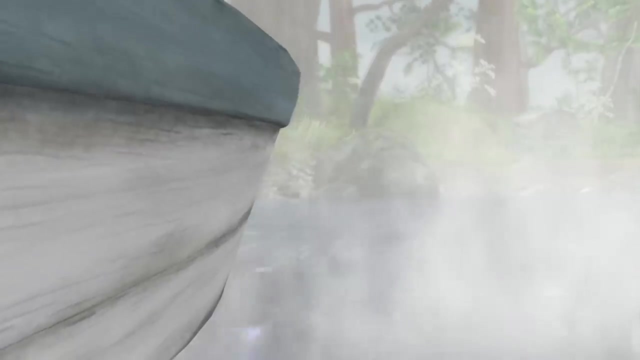 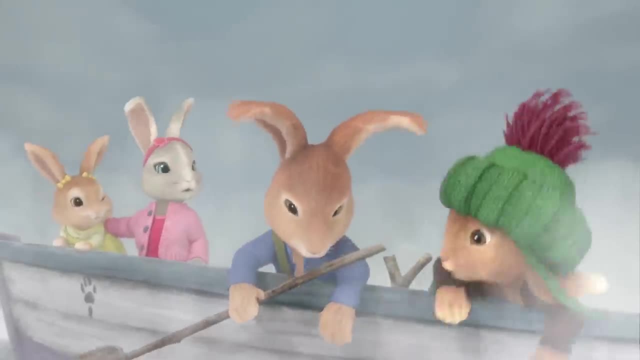 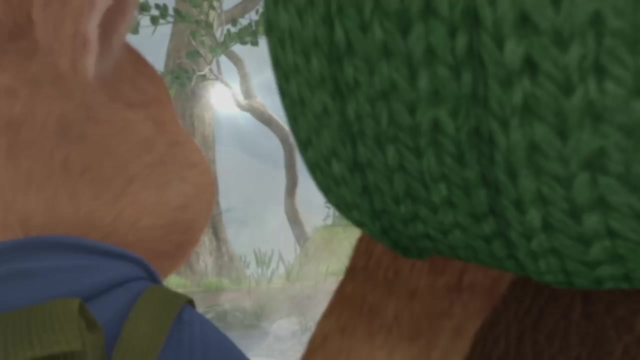 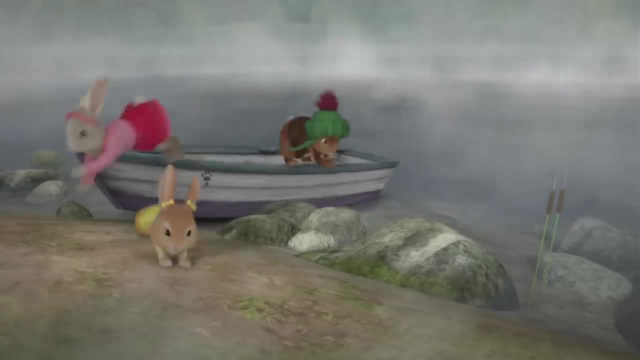 Ah Ah Ah. No wonder it's called Rocky. Ah Ah, Island. Ah, Look Old Rusty's signal This way. Ah Ah Ah, Uhh, Ah, Ah, Ah, Ah Ah. 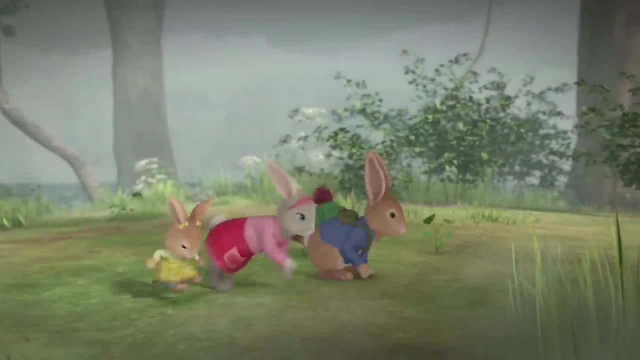 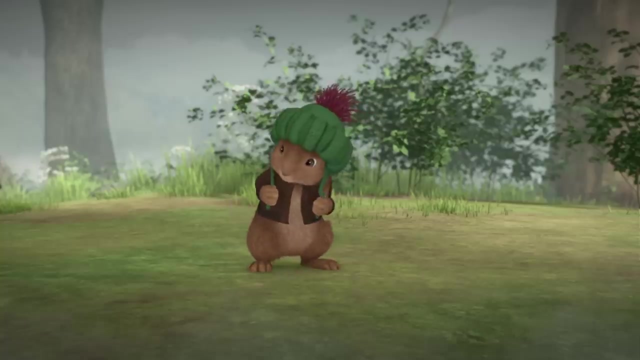 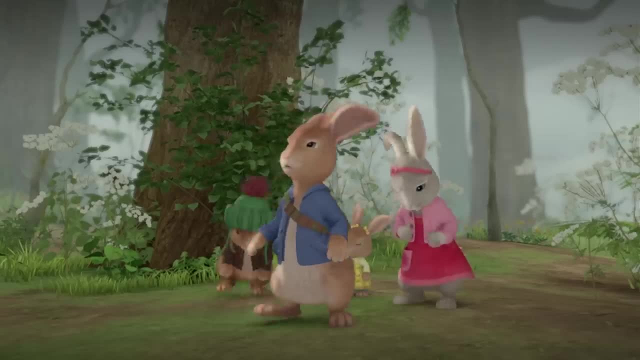 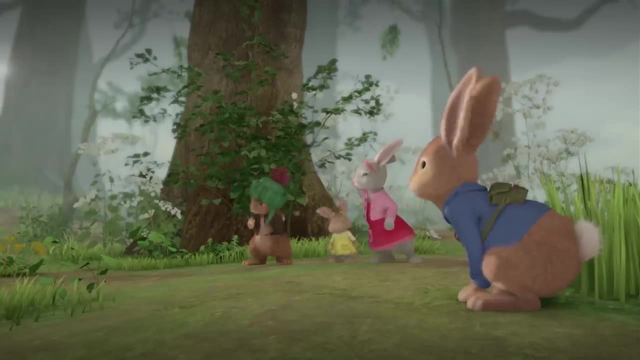 Rub It's a-breve. Are you sure the signal It's coming from over here? Trust me, It's this way, or maybe that way. I ketchuped him again. Roll Oh Uh, Bun Out Ernes. 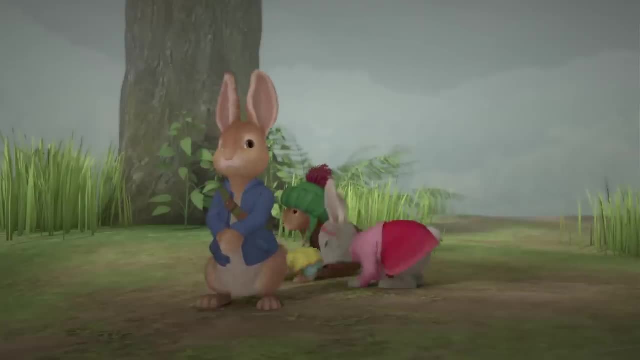 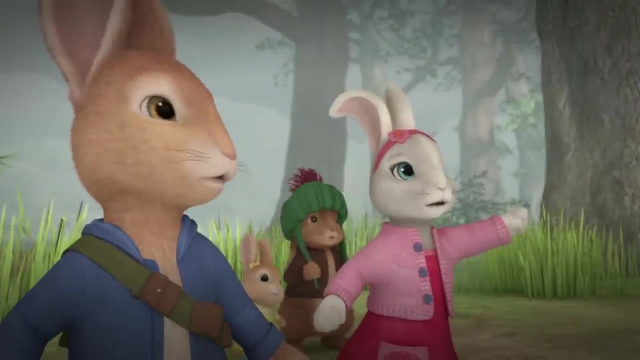 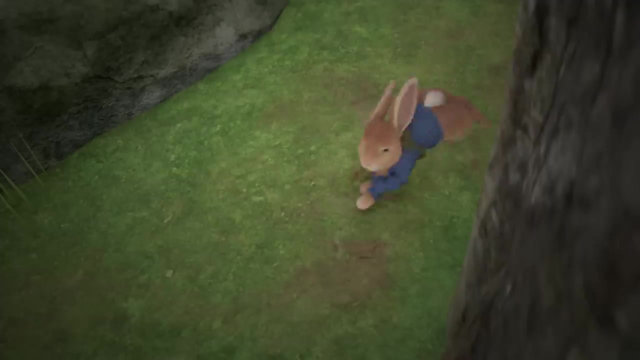 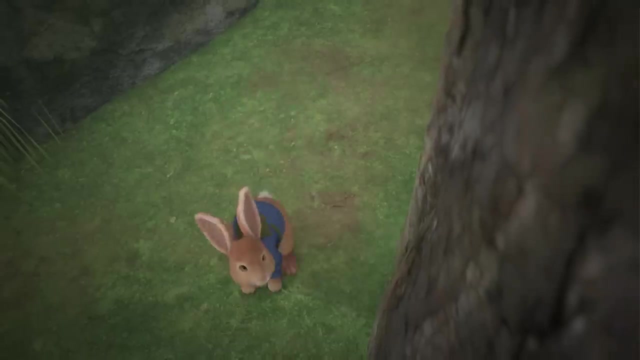 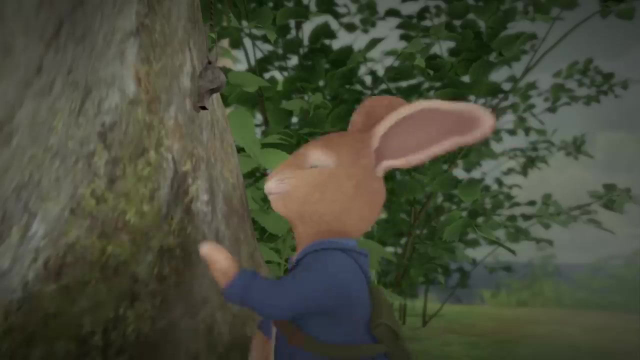 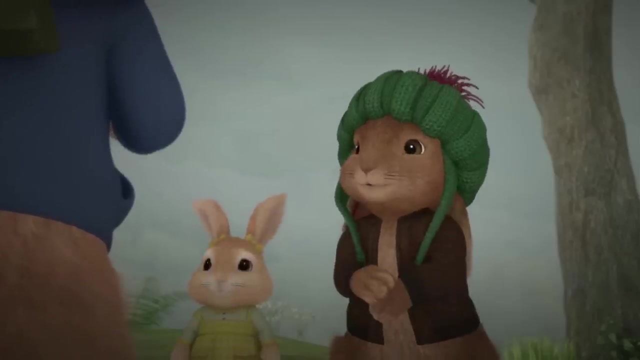 I don't understand. The signal was coming from right here. Peter, Excuse me, Old Rusty, Is that you Hello, Ah, Ah, There's something written on the side. What does it say, Peter, Old Rusty? Loudest whistle in the world. 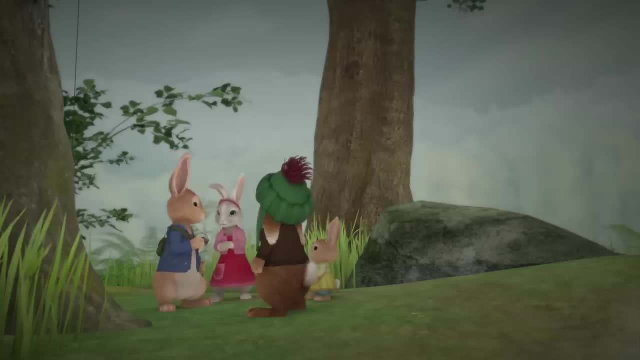 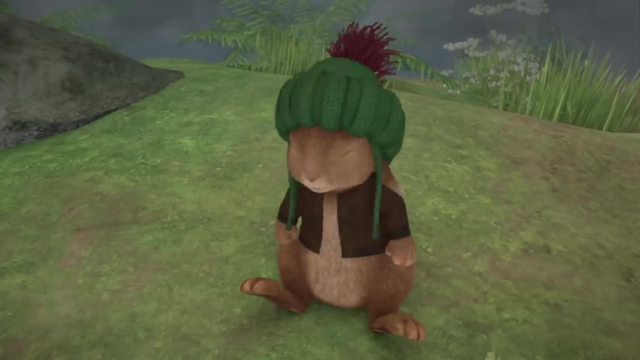 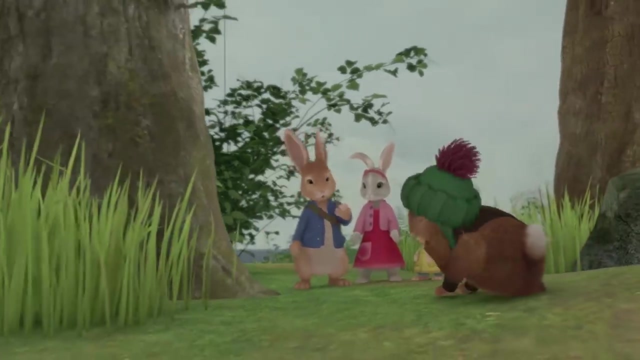 Old Rusty is a whistle lost to the island forever, just like it said in your dad's journal: Ah, Ah, Ah, Ow, Wow. That's even louder than your whistling Lily. All this way For a silly old whistle. 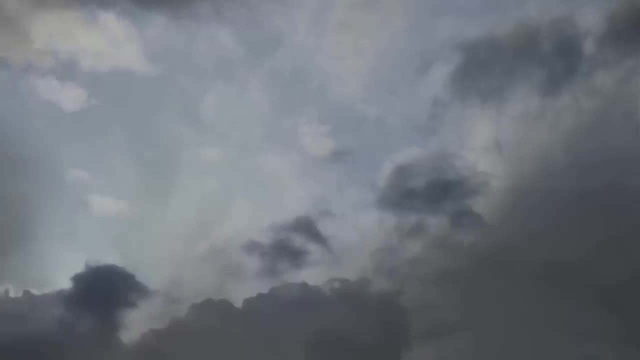 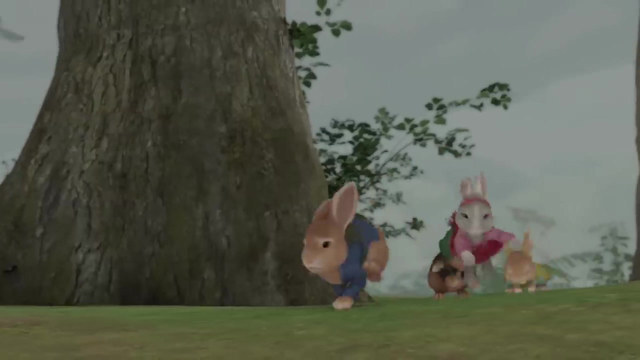 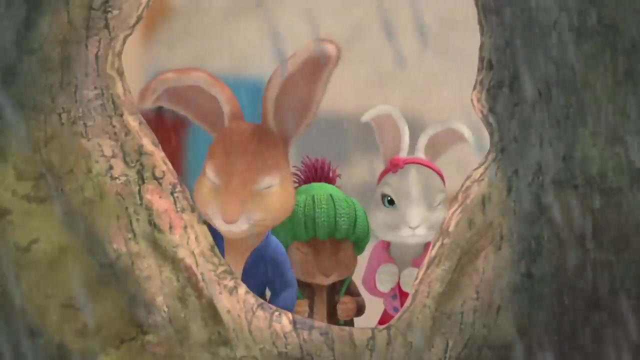 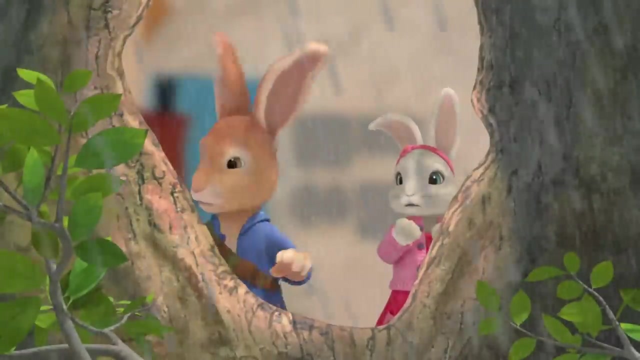 Oh shiny, Oh Oh Uh, I think maybe we should. Storm's coming Back to the boat. It's okay, Benjamin, It's only thunder, I know Whoa. All right, you three, Let's warm you up with some soup. 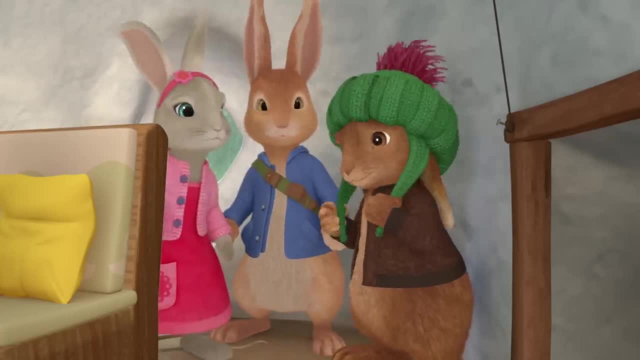 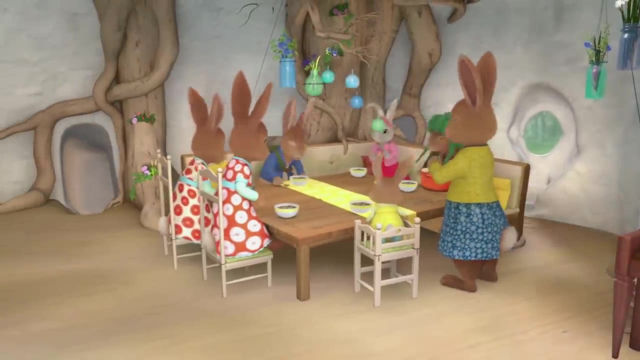 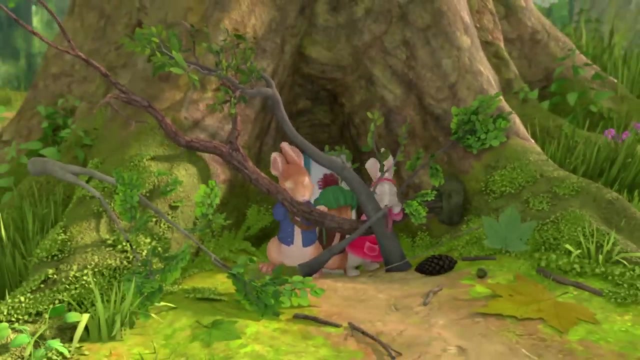 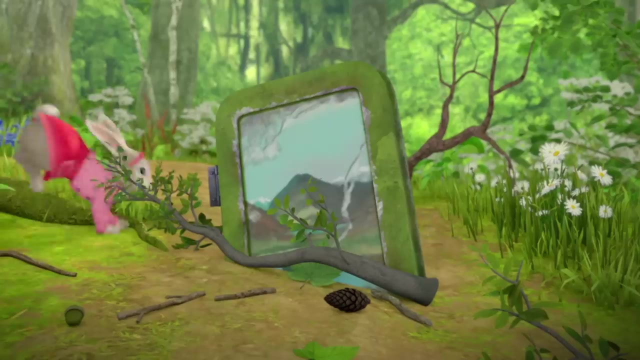 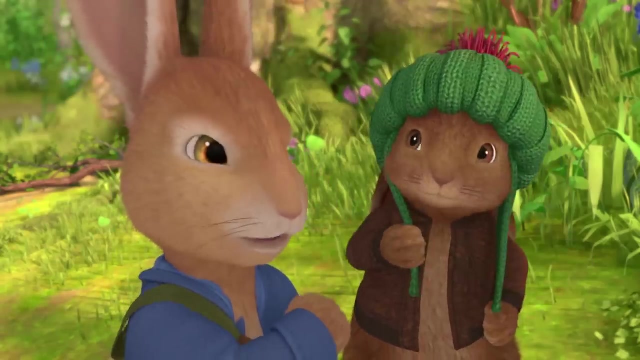 Wow, What a storm. Uh, that was me. this time Storm's over, Come on. Ah, What a mess. Look familiar. It's from our treehouse. What's it doing all the way over here? We'd better go and check it out. 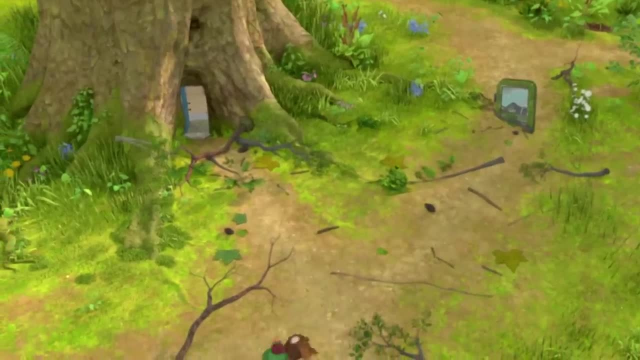 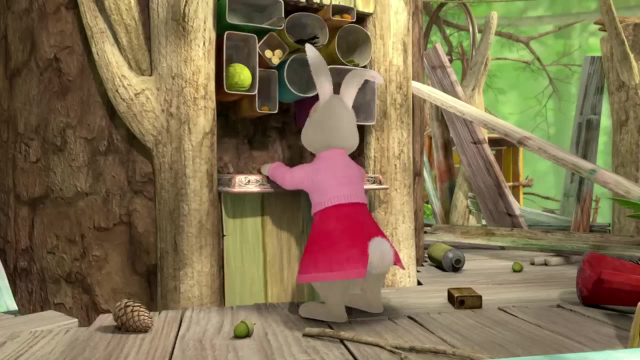 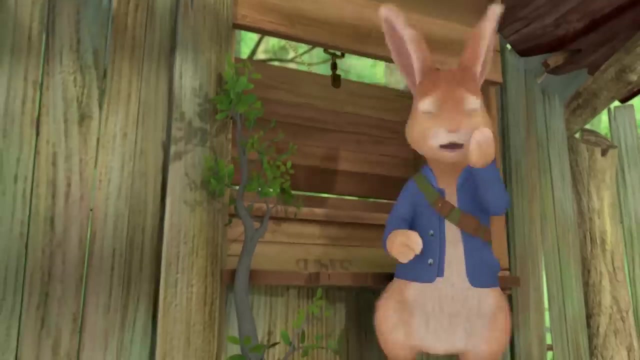 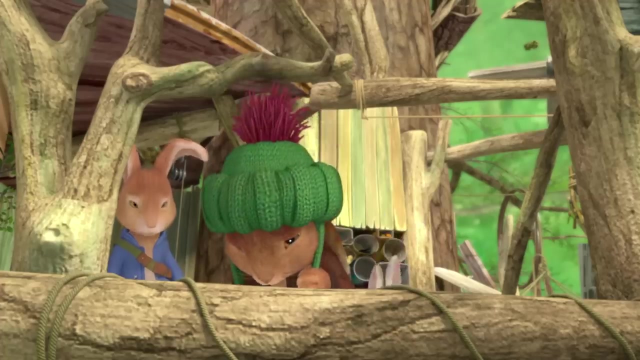 Oh no, Our treehouse. All my drawings are gone. Ah, the telescope's missing too. It's completely wrecked. It's a mess. It'll be okay, Benjamin Hopping hazelnuts, You guys really need to take better care of your treehouse. 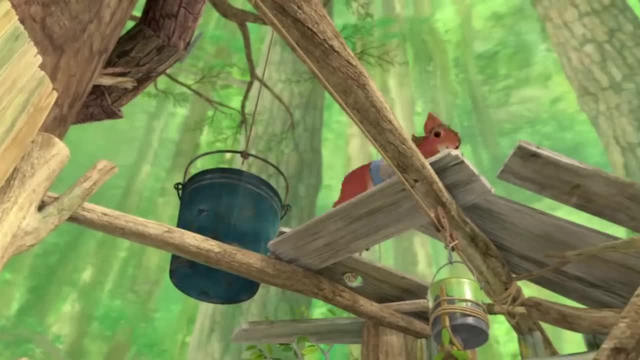 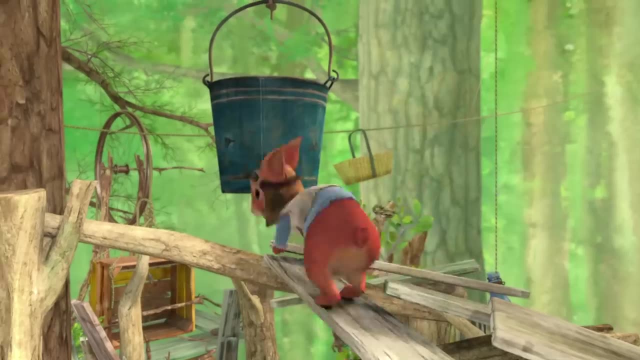 It was a storm, Nutkin Storm, Where I love storms. Sorry it's already happened. Oh, I guess I slept through it. Hey, that explains why I woke up. next to this, Our telescope. There must be pieces of our treehouse all over the woods. 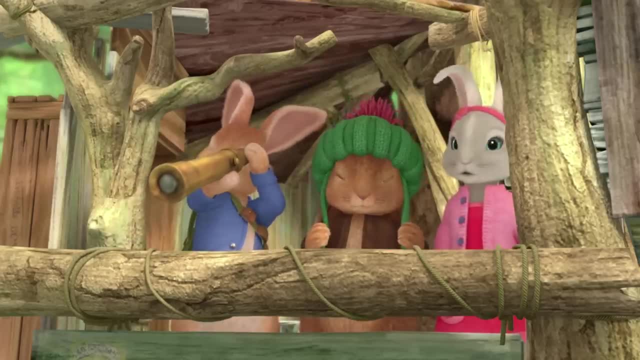 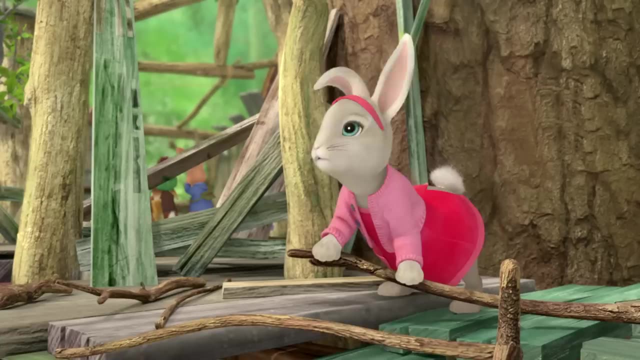 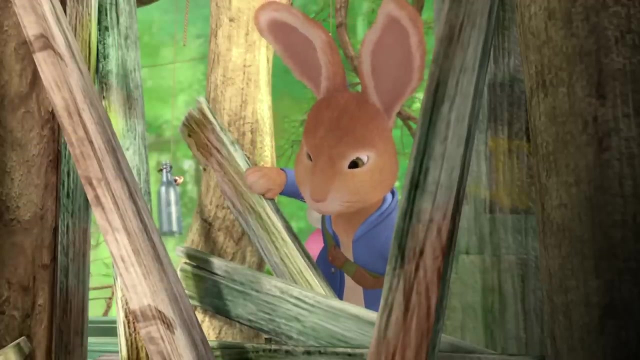 Look, It's a big one. It's a big one. Look, Tommy Brock's got some of our roof. Do you know what else is missing? Your dad's sign, Huh, Oh no. What are we going to do? 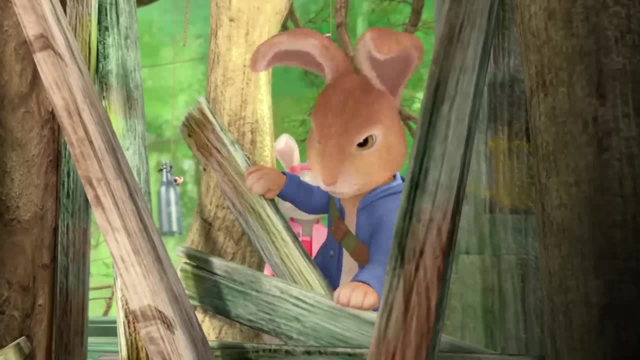 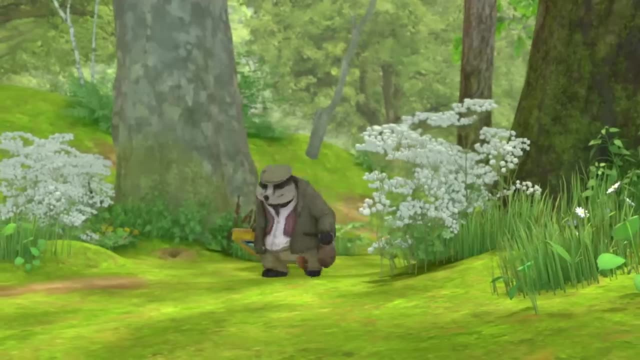 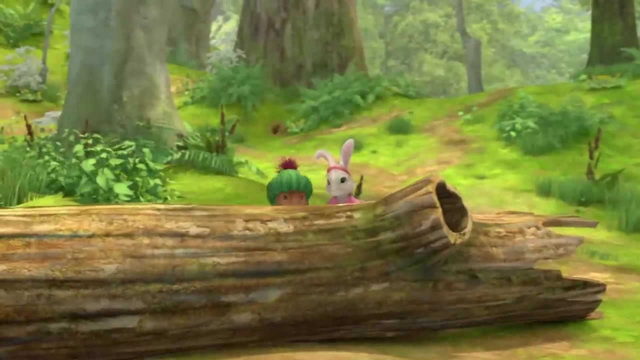 There's only one thing to do. We're going to find every single piece of our treehouse, starting with that roof. Let's hop to it. Oh, I do love the wind. It blows things around, Except the pieces I find on the ground. 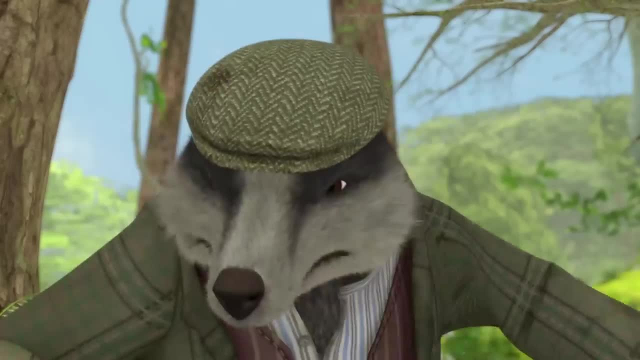 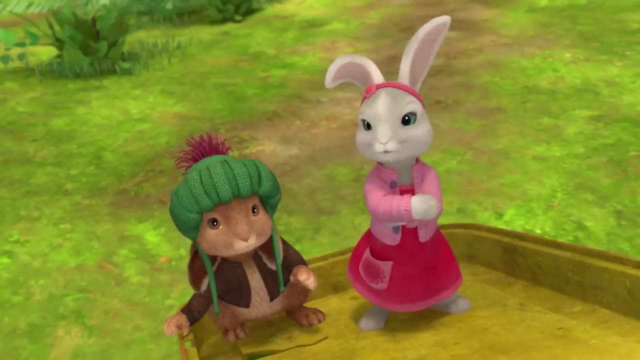 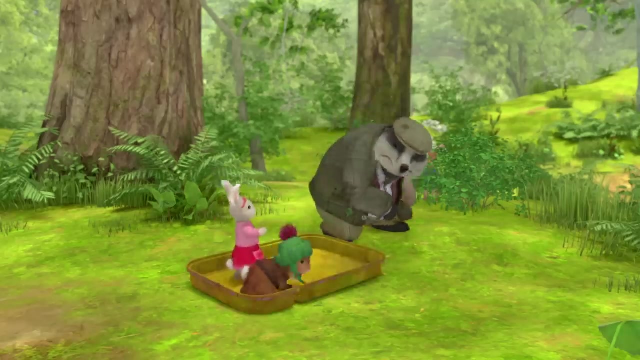 Huh, Rabbits, Get off my tin. No, can do, Mr Brock. This tin belongs to us, Isn't that right, Benjamin? Yes, I mean, uh, Yes, I don't care, It's mine, now Stop. 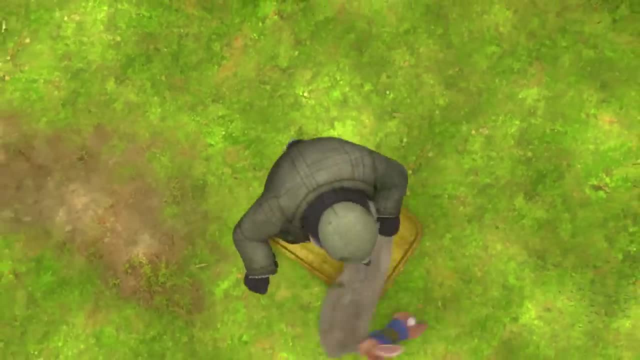 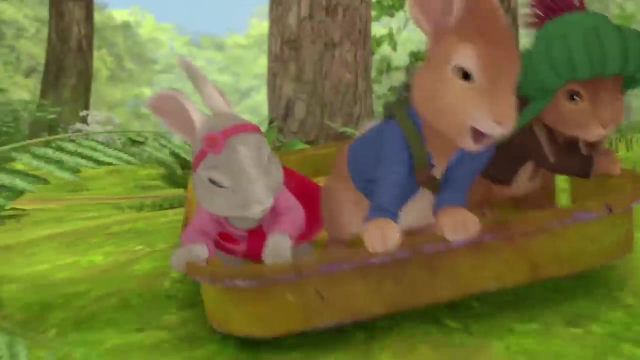 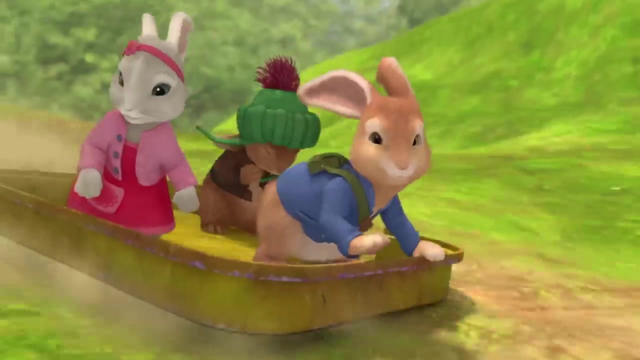 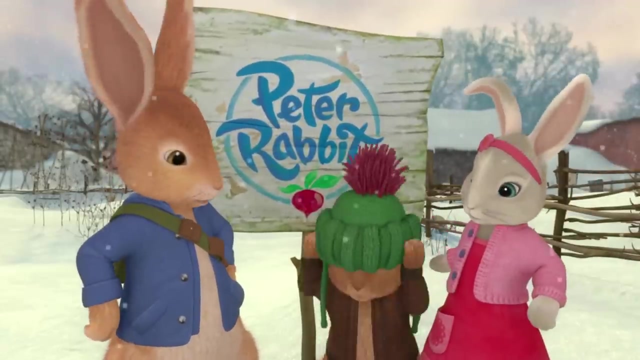 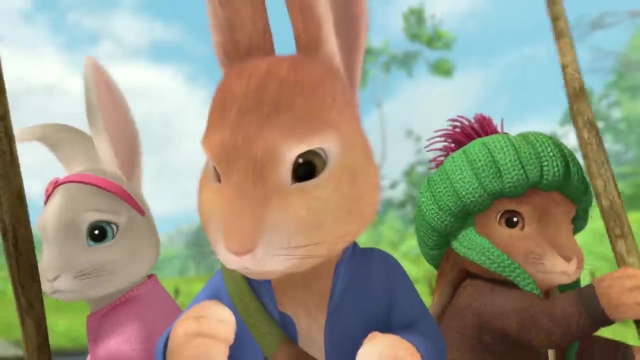 Stop. Sorry, but our treehouse needs its roof back. Yee-haw, Hop back here. I'll turn you into a fur hat. Hey, The raft. I'll take you to the raft. I'm going to get you out of there. 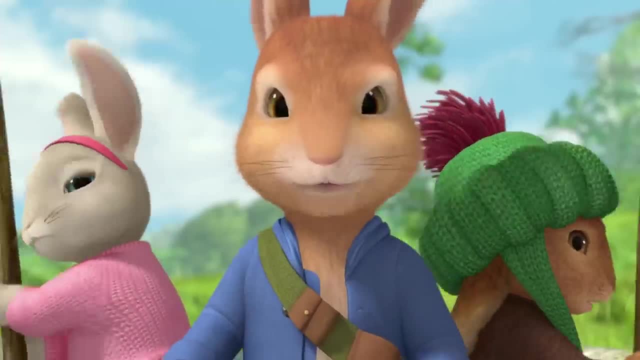 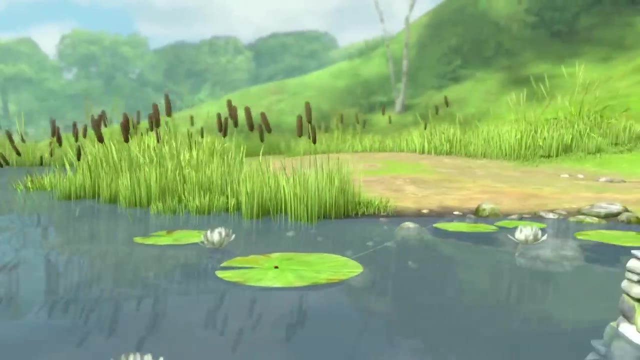 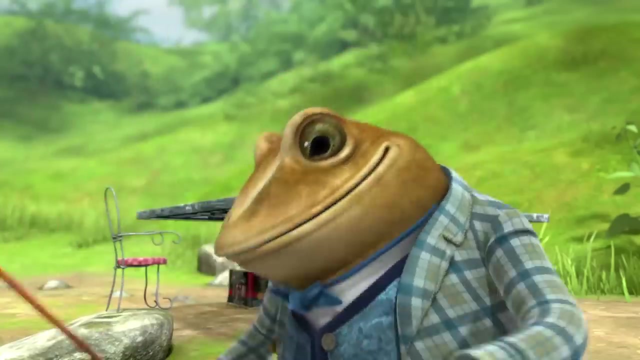 OK, I'll tell you what I found. I don't know what it is. It's a little. Hmm, I know what it is. It's a little. I don't know what it is. I don't know what it is. 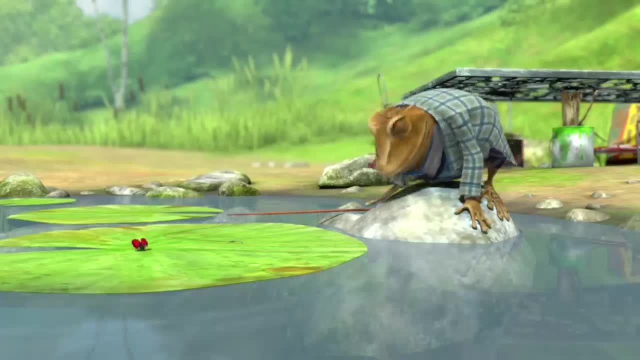 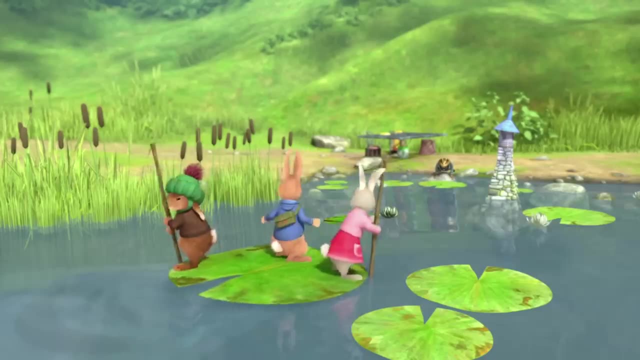 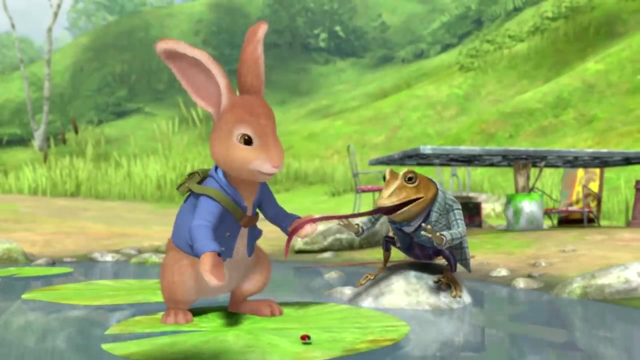 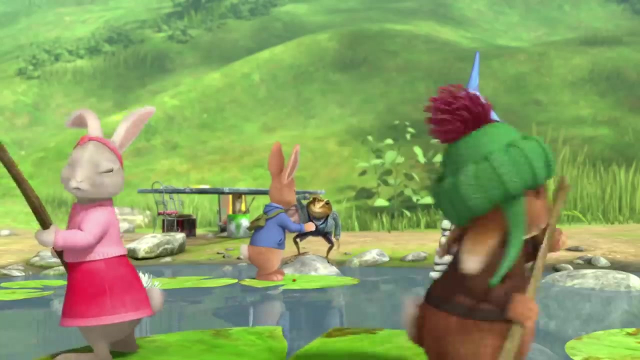 It's a little. I don't know what it is. It's a little Wrong way, Benjamin. Sorry, Mr Fisher. Florence isn't just a bug, She's a friend. Tell me, Florence. Hey, I think I'm getting the hang of this. 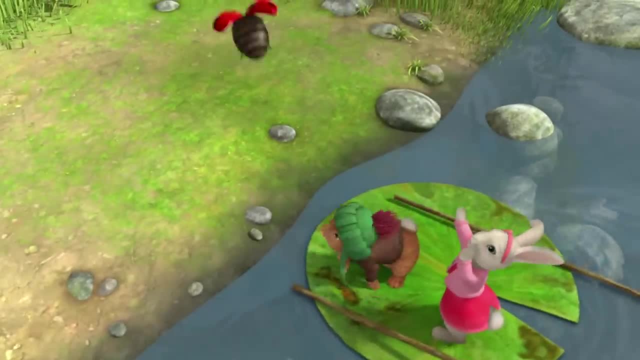 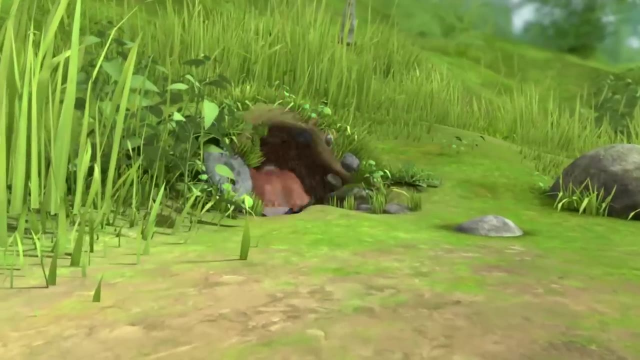 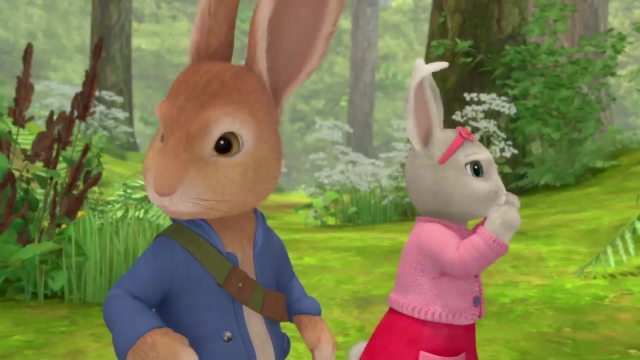 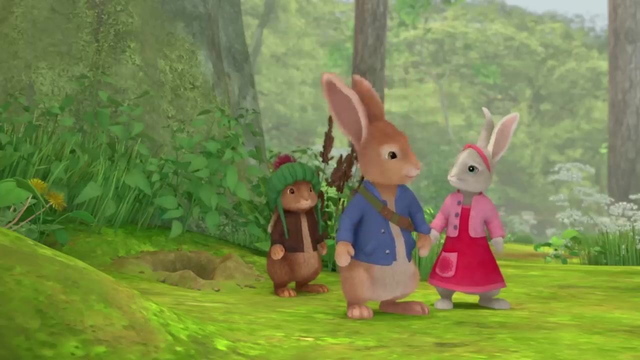 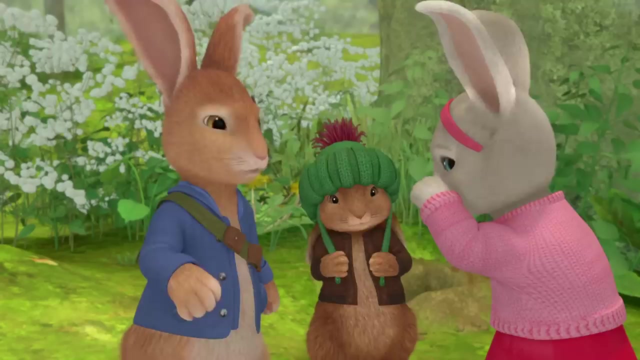 There she goes again. Florence, Florence, Florence. She went this way. I think I wish you'd just kept an eye on her, like you'd promised. Lily's right. This is our fault. We'll get her back, I promise. 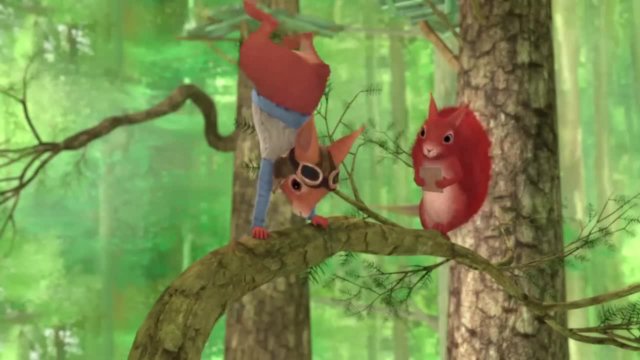 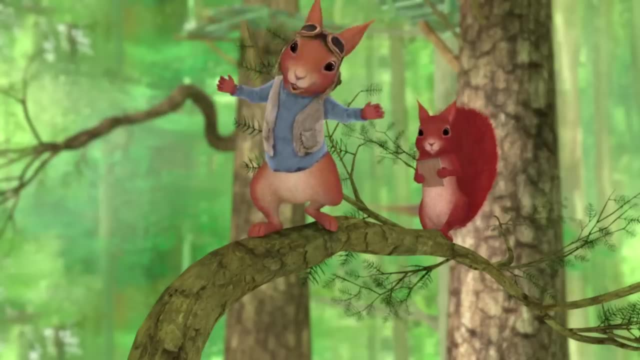 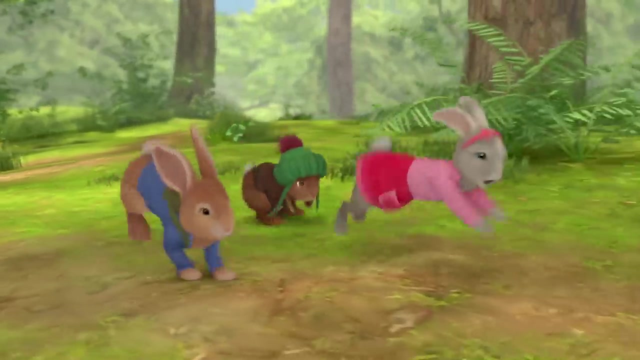 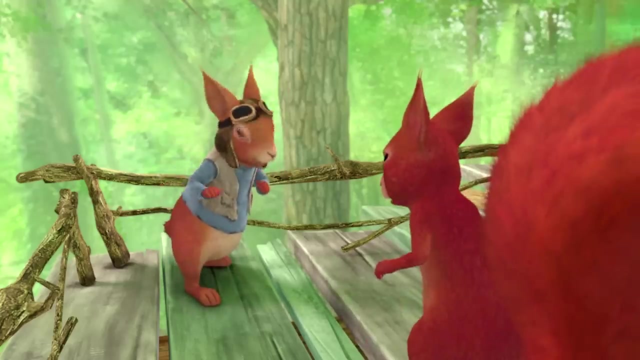 1,048! 1,049!. Have I beaten my record yet, Felix? I'd know that whistle anywhere. I don't see her. Oh, Florence, Please come back. Lower the platform, Felix. Our friends need us. 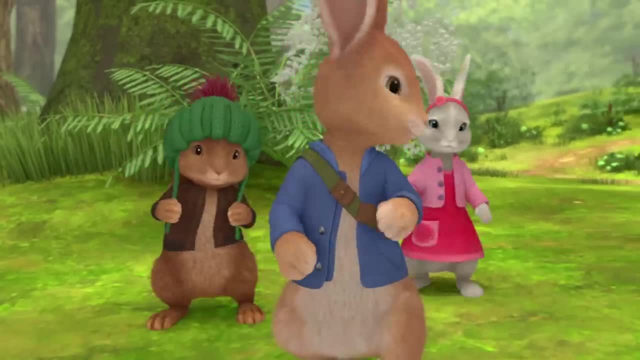 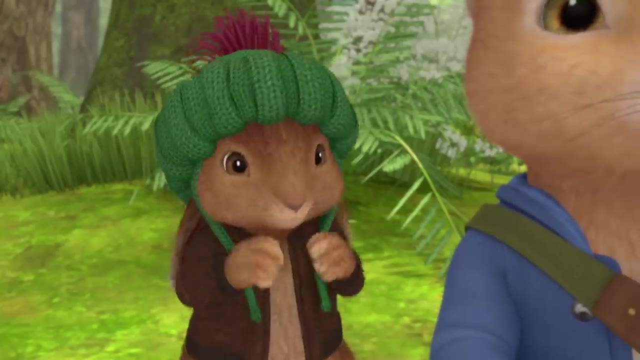 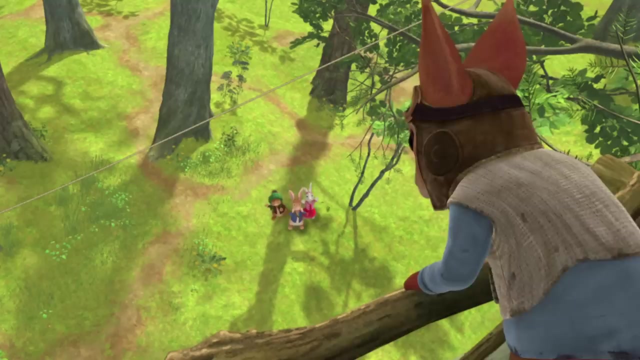 There she is, Florence. We've found her. Three cheers for us, Hip, hip. Oh no, Look, She's going to get squashed. Stop, What's that you say? Stop, Stop, Drop your thing. 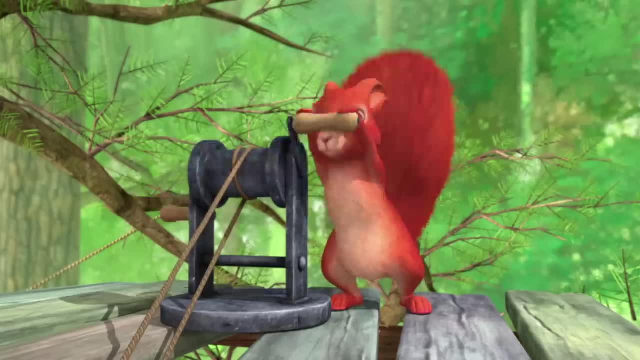 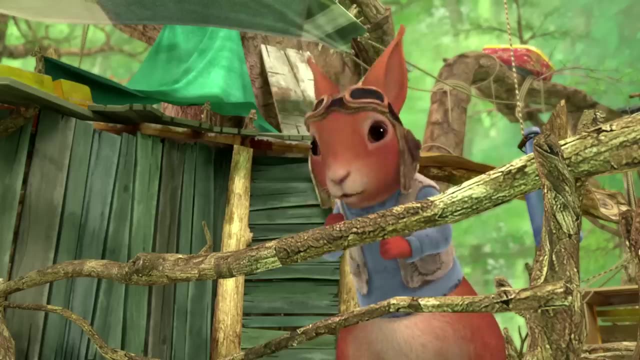 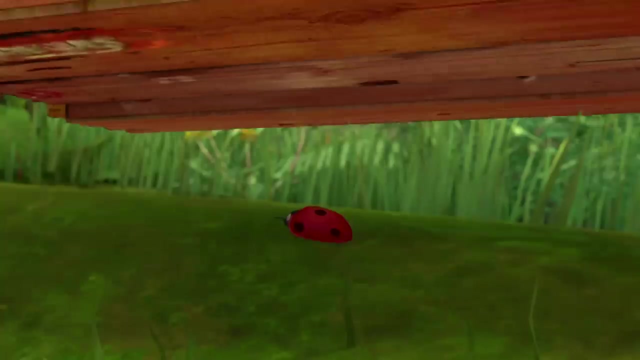 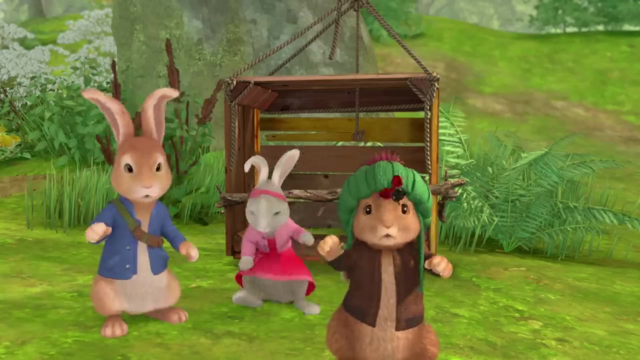 Master, Felix, put your bag in the bin. Stop, It's so good I can't hear you with all this noise. Felix, stop it, would you No? Up Nuggin, put us up. Felix, you heard them. 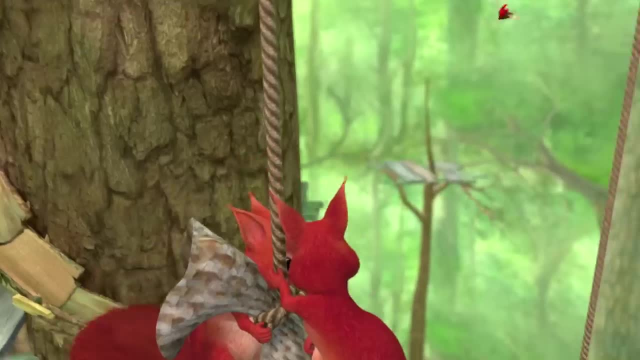 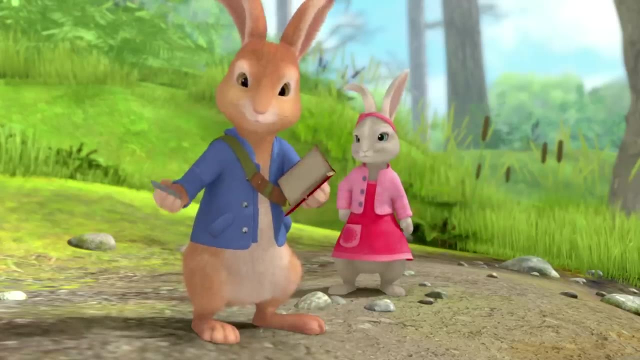 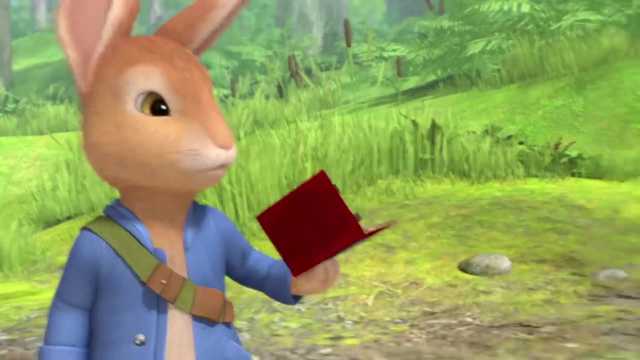 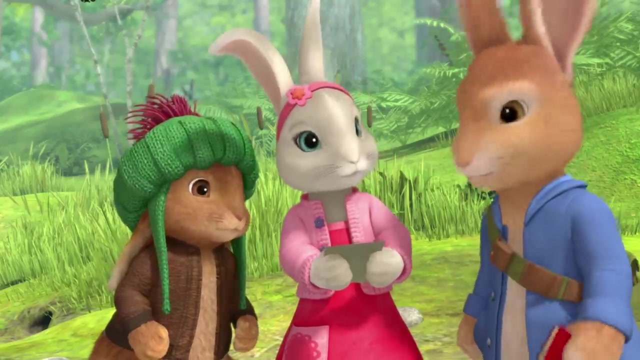 Up. Let me show you. OK, Flat arm, loose wrist, pull back. That's what I did. Huh, Wait, What's this? I thought I'd read every page of my dad's journal, But I never saw that before. 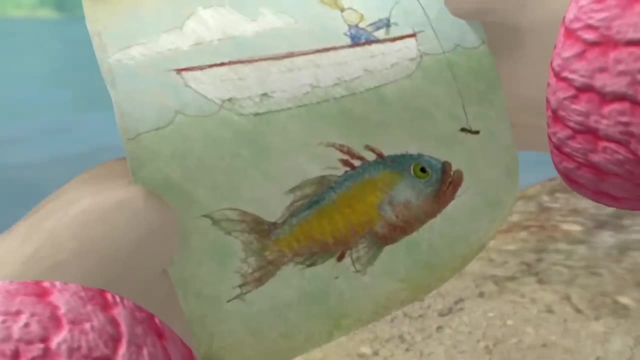 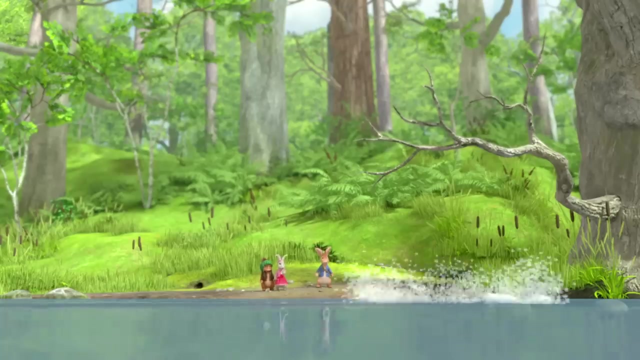 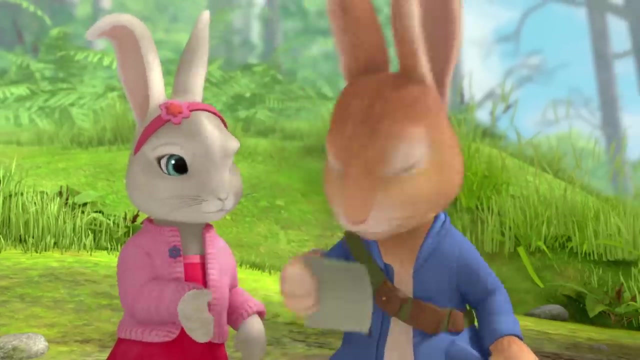 That's a big fish, A really big fish. Wow, The biggest fish I've ever seen. Whoaaa, What was that? It's the same fish as the one in the drawing And it's right here in this lake. Maybe fishing isn't such a good idea after all. 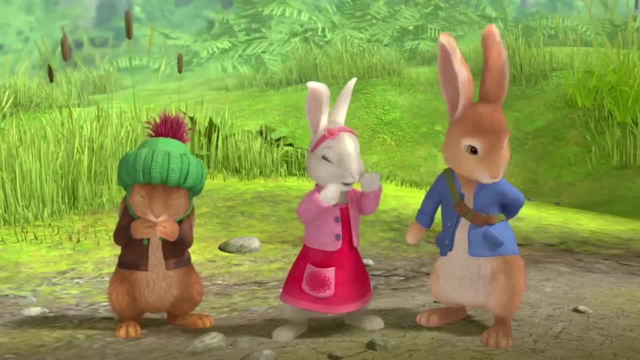 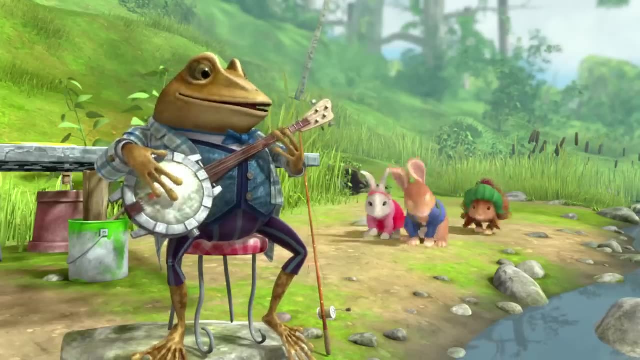 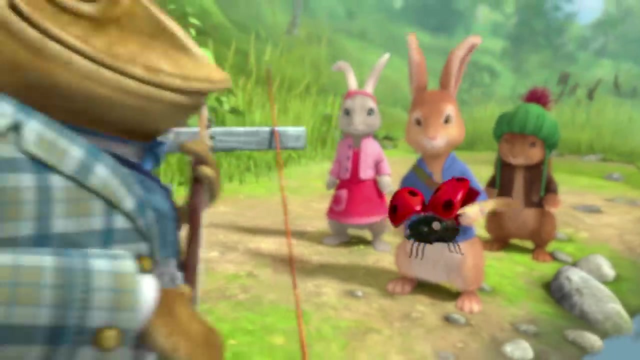 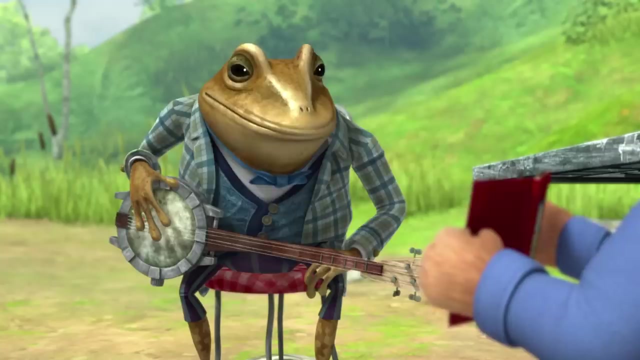 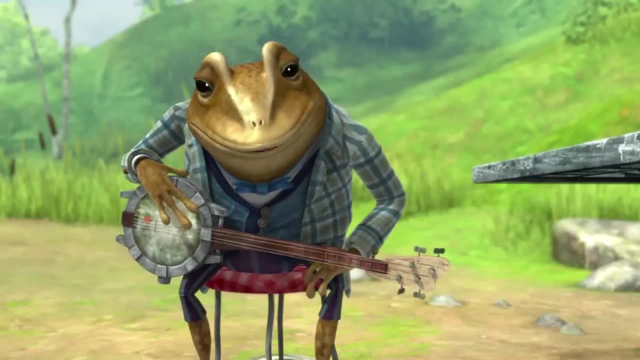 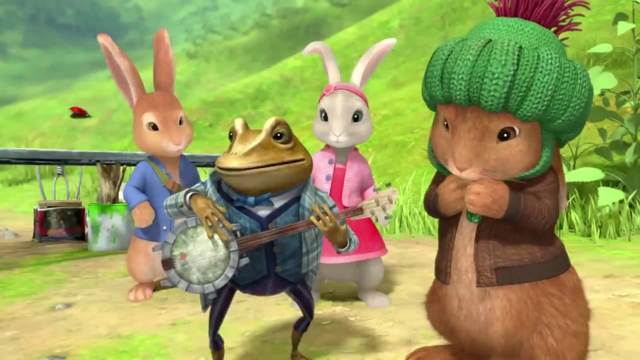 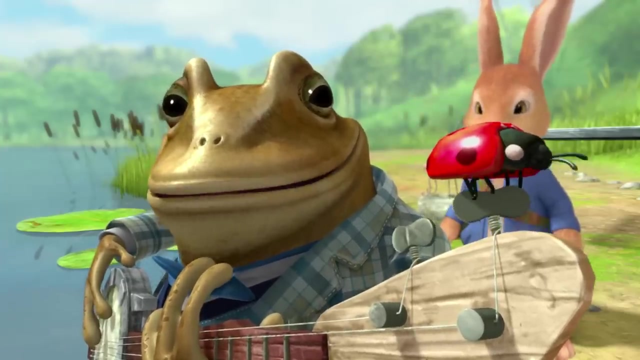 It's the reason why I don't go far out on the lake anymore. Who is he? The meanest, strongest, nastiest fish of all. No one has ever come close to catching him Except- Oh no, you don't. 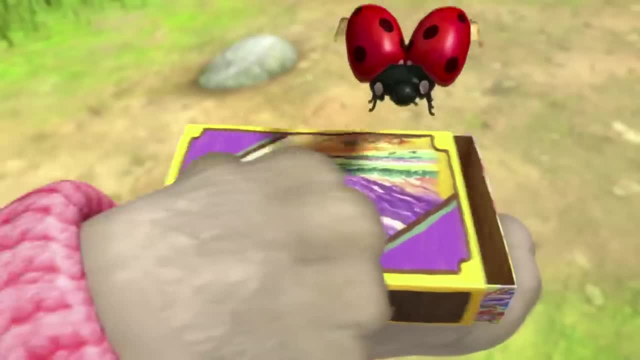 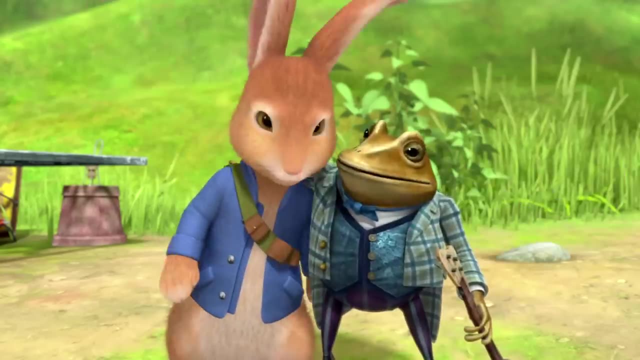 Yes, Mr Fisher, no one except. Where was I? Oh, yes, No one except your father, Peter. One day he was out fishing and he came face to face with- Oh no, I can't say his name. 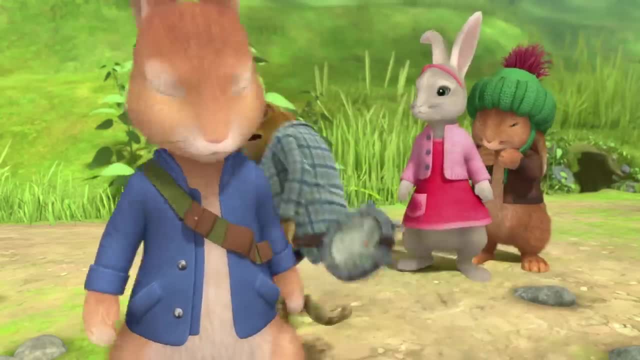 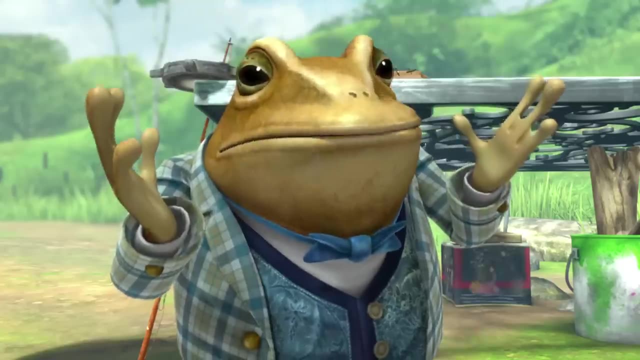 Please, Mr Fisher, tell me his name. Oh no, I can't say his name. Oh no, I can't say his name. Tell us Jack Sharp. The fish is called Jack Sharp. There, I've said it. 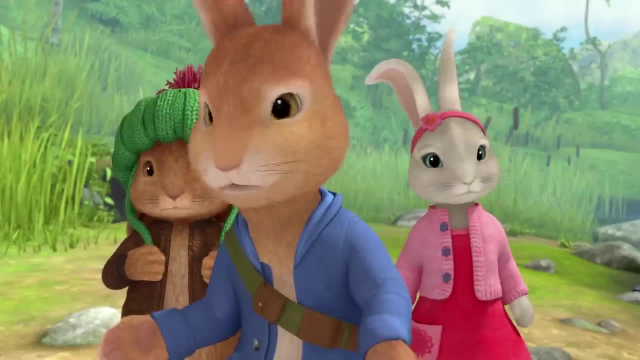 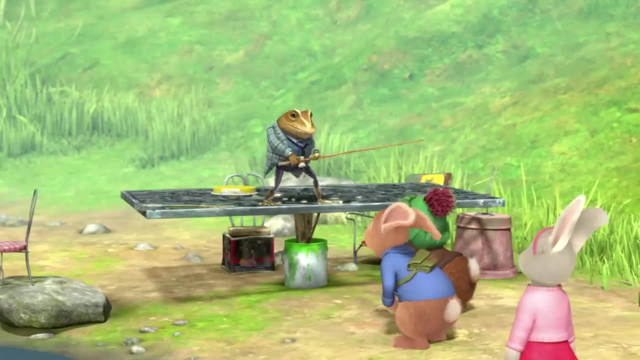 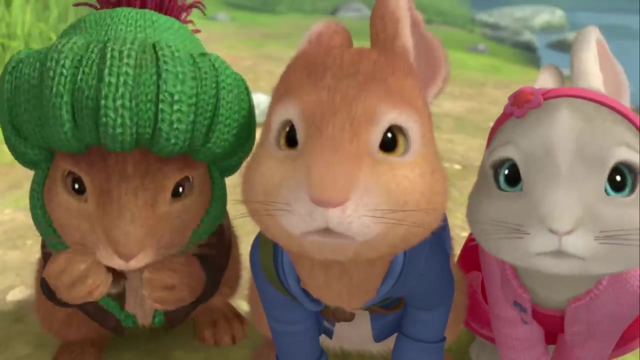 So what happened? How come this Jack Sharp is still in the lake? Your father was determined to catch him. He cast his line, Pulled to the right, then the left, then right again. Suddenly he lost his footing, But so big was Jack. 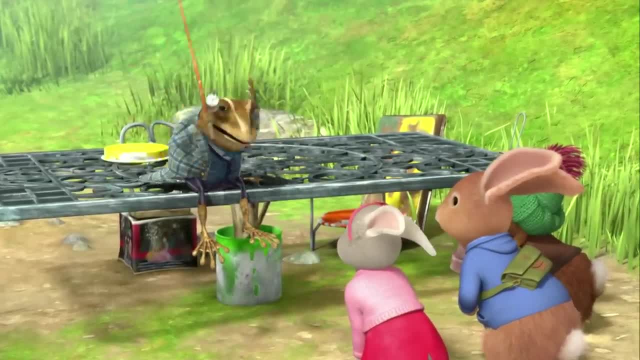 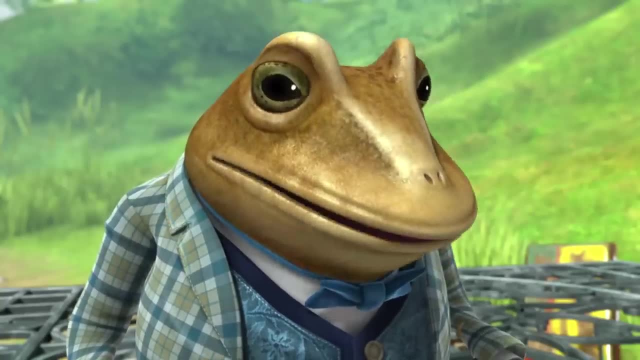 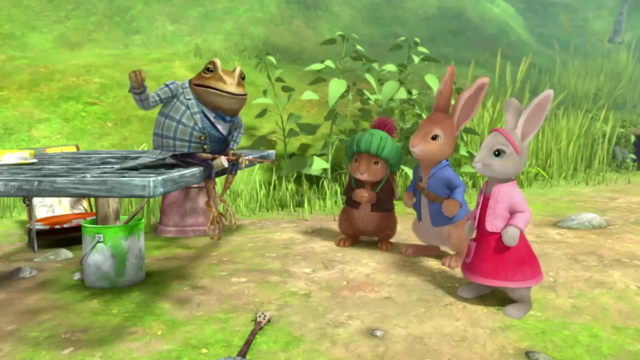 that he was too much for a great adventurer like your father to reel in, And And I went for help. But when I returned, Jack Sharp was gone And your father never spoke of the great fish again, And from that day I called Jack Sharp. 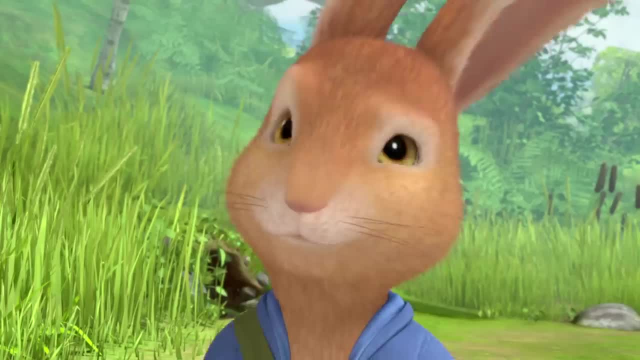 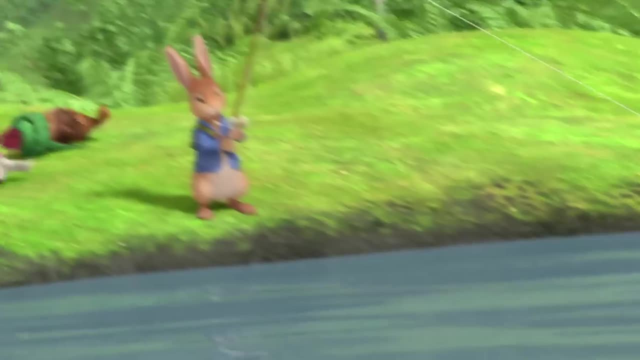 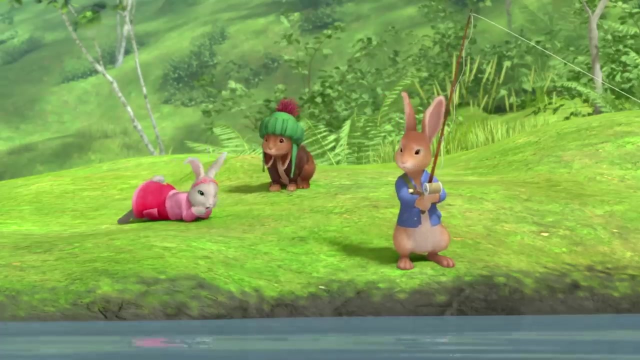 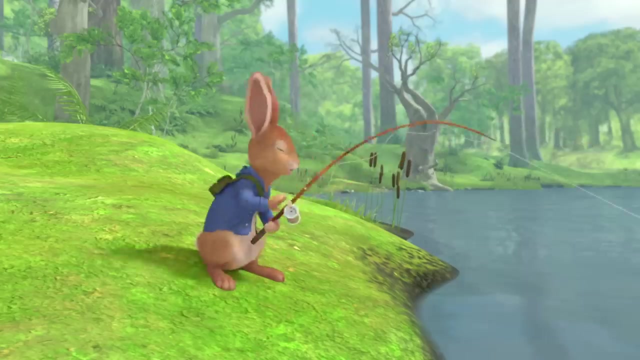 the one that got away. Can I borrow your fishing rod please, Mr Fisher? Maybe Jack Sharp is asleep or something. Maybe you should try wiggling the rod. Nothing, Can we go home now? Wait, I think I've got him. 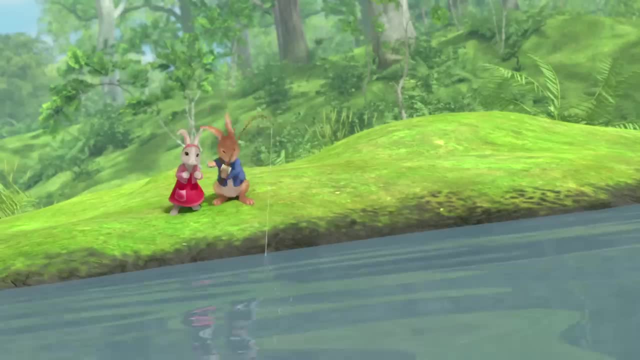 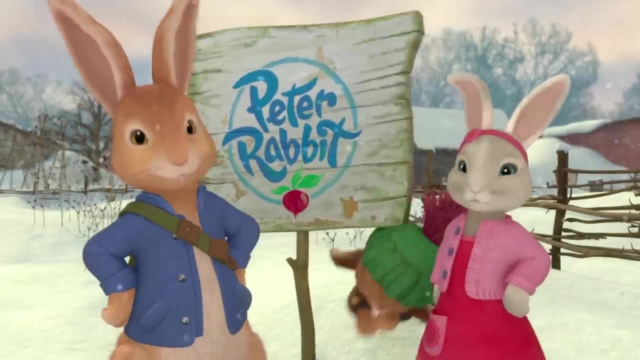 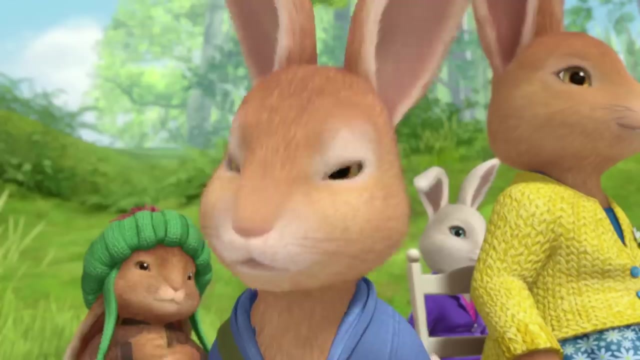 That's him Run. Well, at least we know the rod works, Mum, I think I saw Mr Todd's tail in the reeds For the last time. Peter, stop telling Fibs, But I'm not. I Shh No talking during the performance. 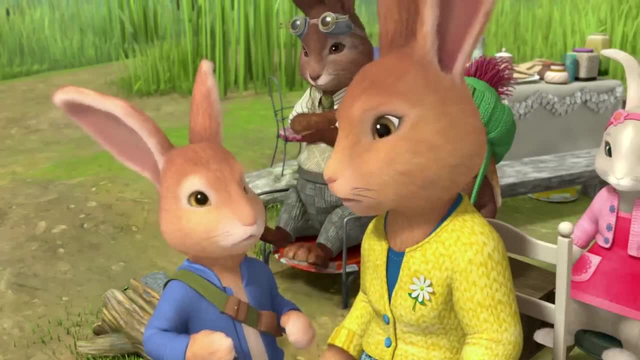 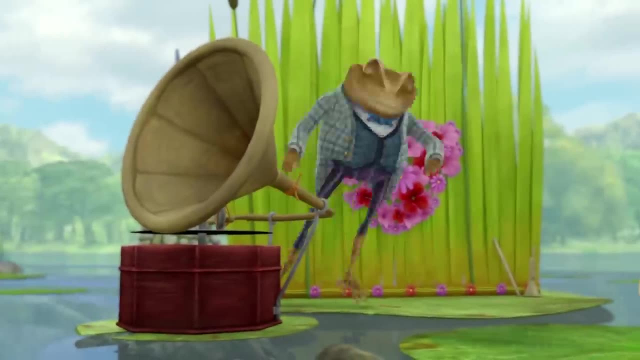 And now for my grand finale, a selection from my days as a ballet dancer Or a dance-movie dancer. Oh yeah, CHOIR SOBS And a great date for theinchy-quinchy. All right, I don't want to talk. 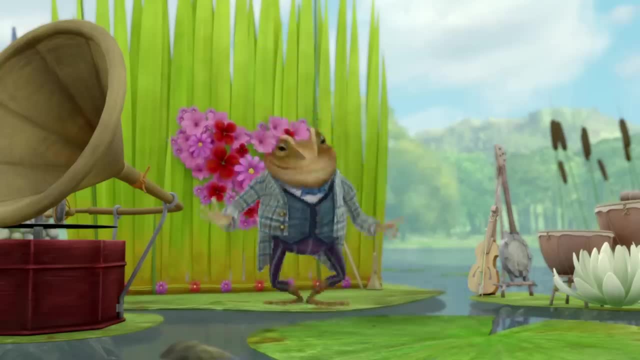 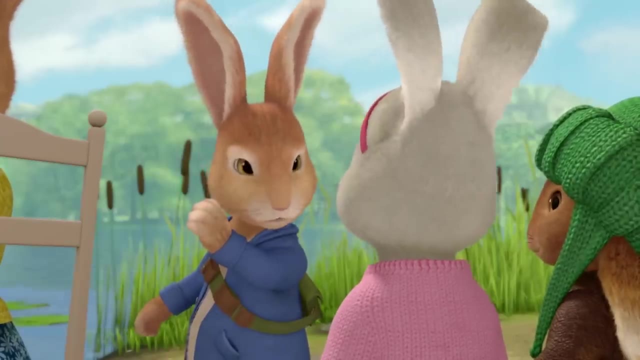 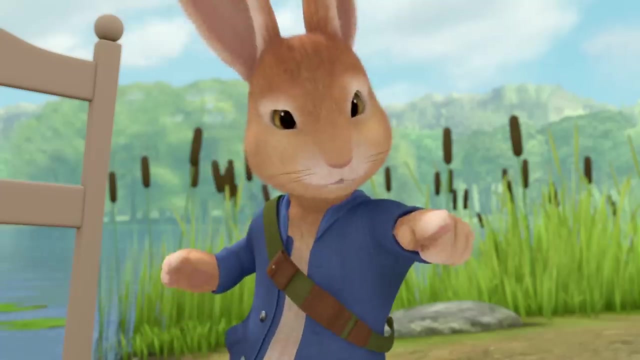 I want to enjoy this bit. OK, Always had good legs, you know. Hey, listen, I think I saw something in the reeds What? Just keep your eyes peeled for that sneaky fox. Oh, no, Exactly, How did you know? I was going to say fox. 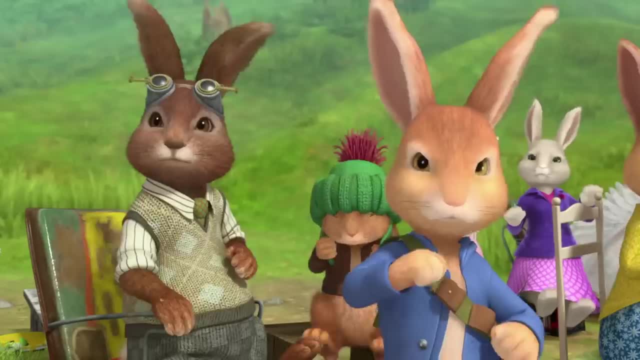 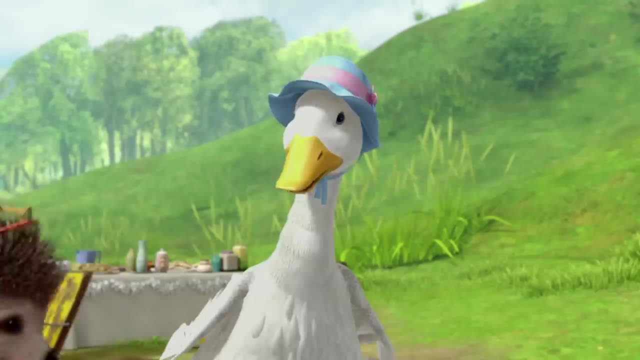 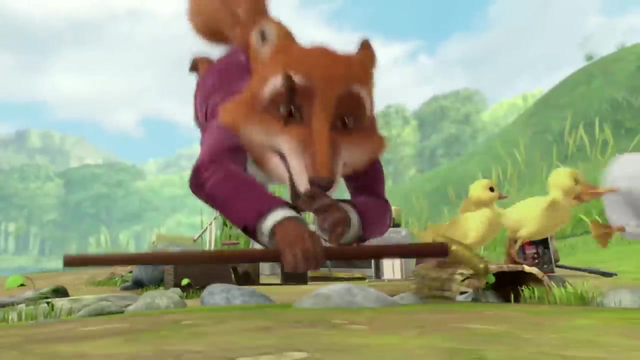 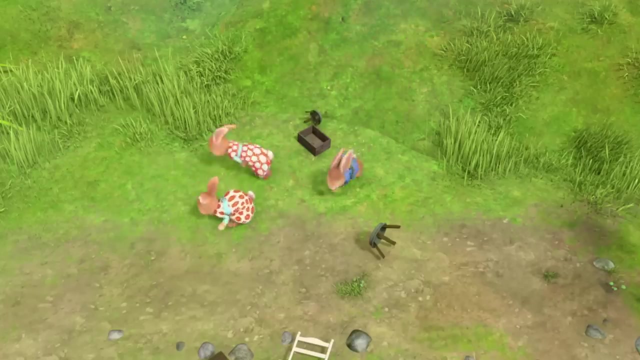 So what's good to eat around here? Run for the trees, Oh no, Oh Mag. Is this part of the show? Oh dear, it's not. This is the funniest thing I've seen in ages. I'm too young to be eating mobs. 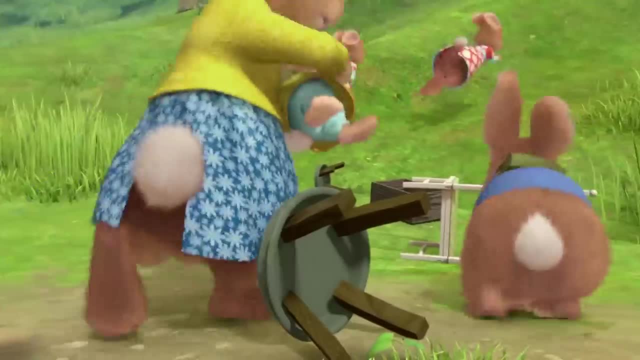 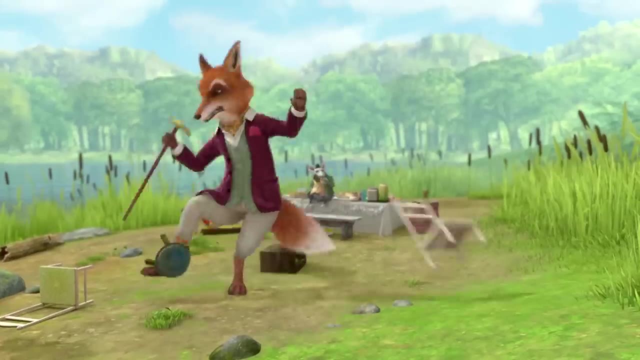 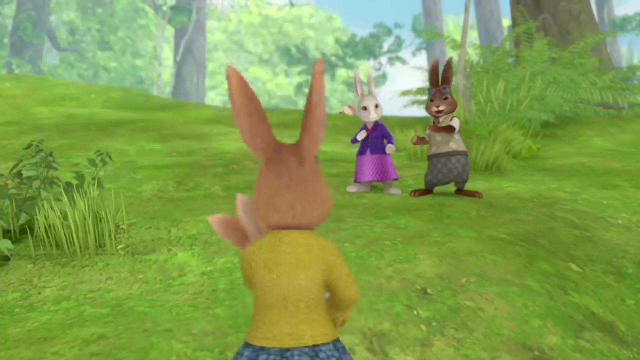 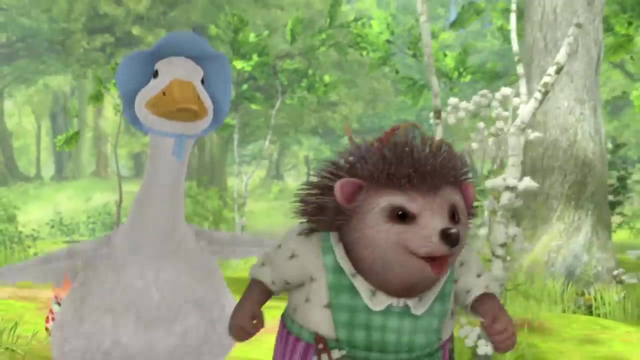 Everyone back to the woods. Come on, girls, Peter. Whoa nice move. Mum, Take that Hi-ya. Peter, hurry, Let's go. Benjamin, You too, Lily, Fast. Look my spats- The nerve of that fox. 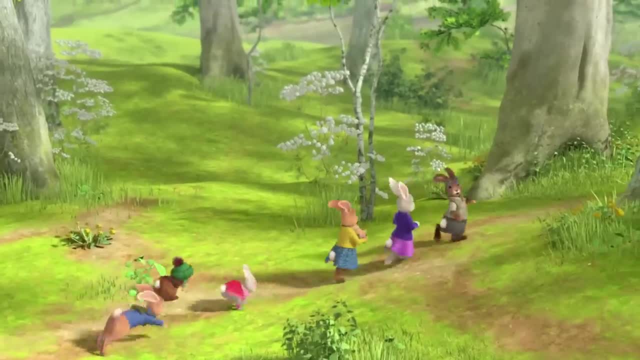 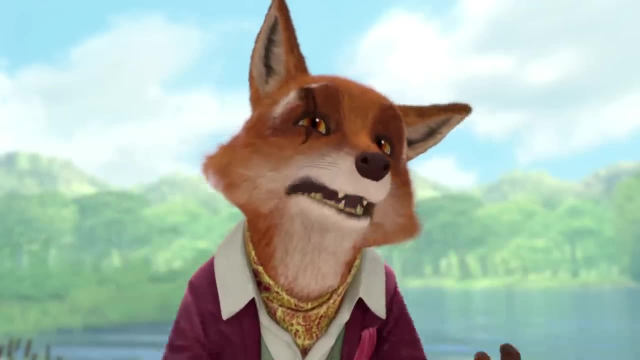 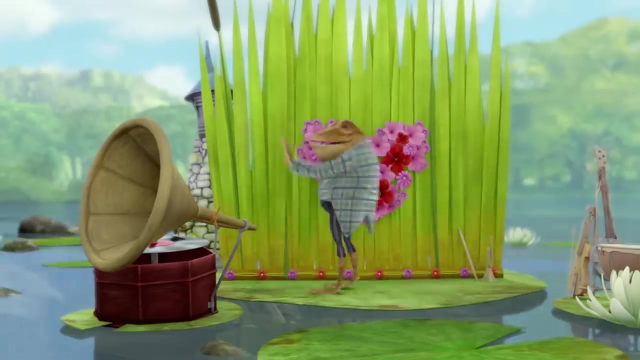 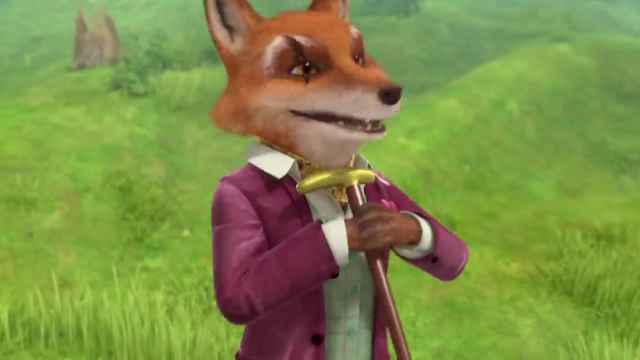 I doubt he was even invited. Come along, Come on now. No, no, no, Everyone's escaped, Not quite everyone ∑. As it happens, I do have a delicious recipe for frogs' legs. Mr Fish is in trouble. 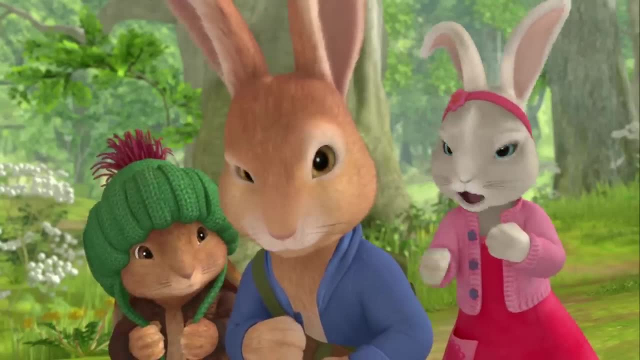 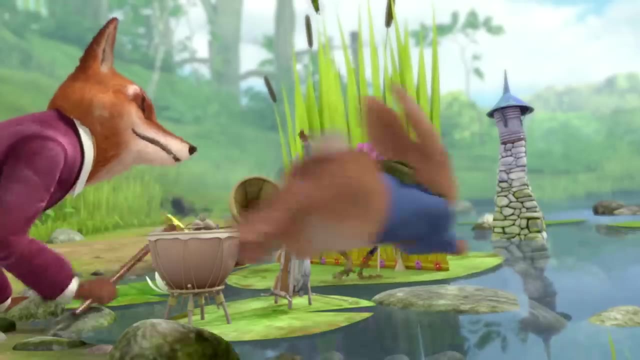 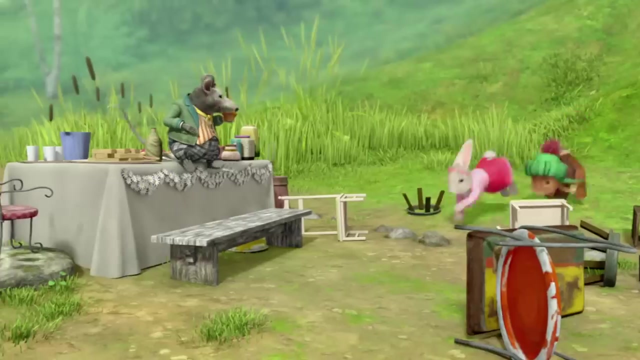 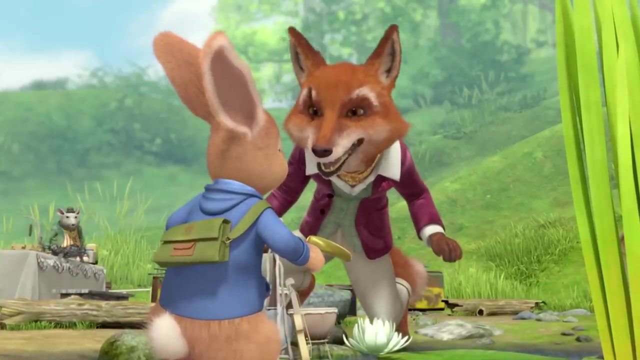 Herzl: a la la laa. Hungry foxes eat frogs. I know that for a fact. Fundory Sapplee Sean away. Zzzz, What, Oh what? back off mr Todd, always playing the hero. sadly, it looks like this will. 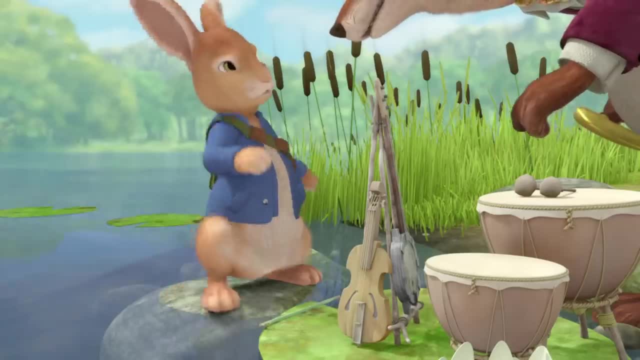 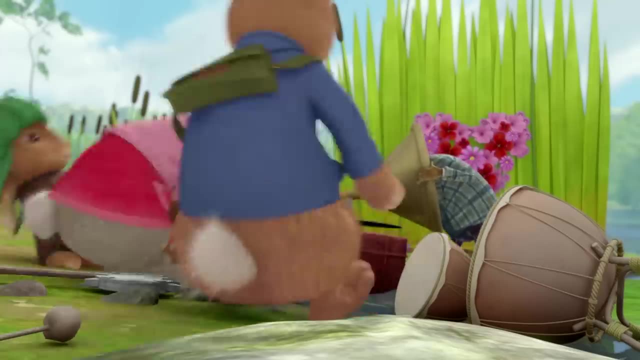 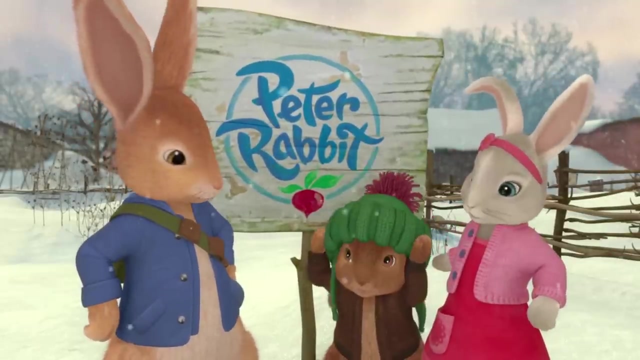 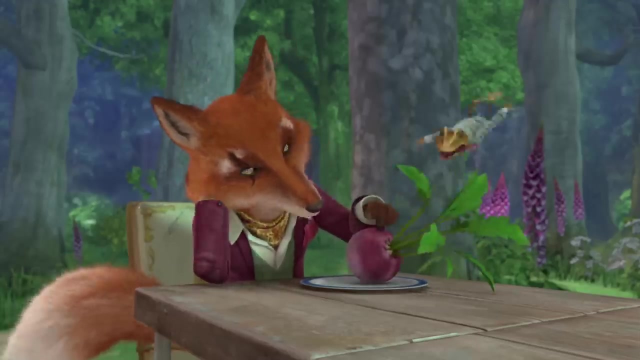 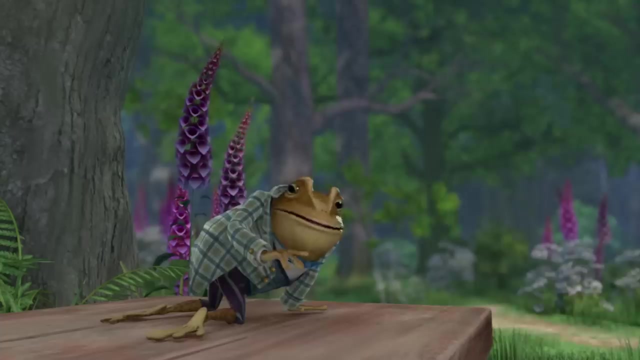 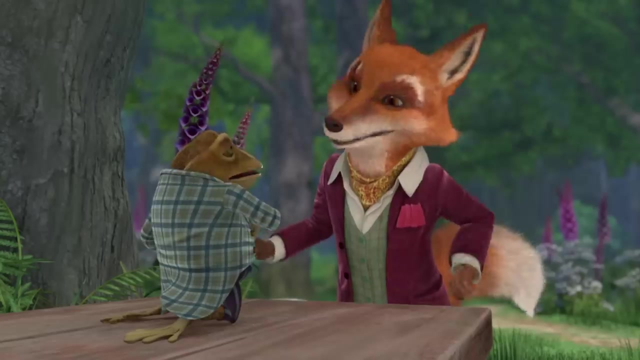 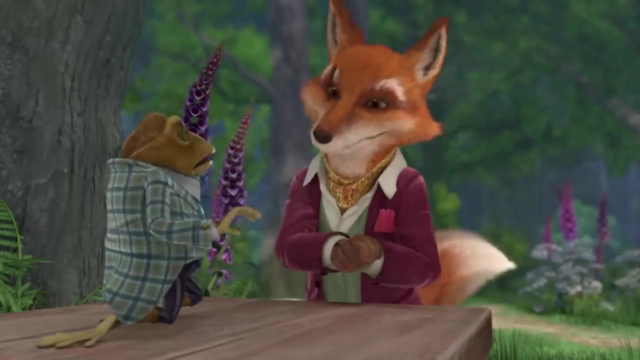 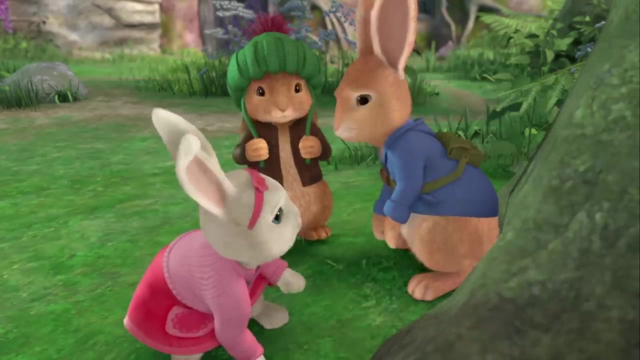 be your last performance. turn it for lunch again. how I wish I had meat, oh dear hey. terribly sorry to intrude, mr Todd. I hope I haven't spoiled your lovely picnic. on the contrary, you've improved it. not again. we'll never rescue him this time. a good rabbit never gives up. we. 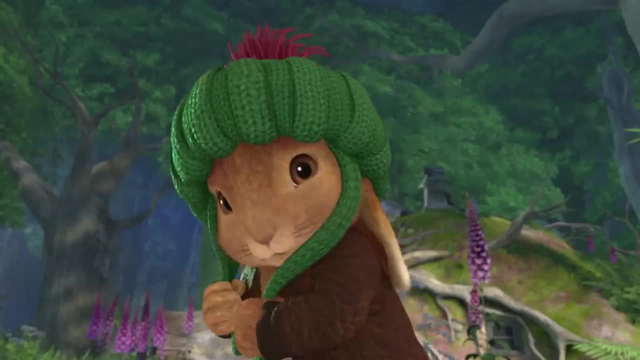 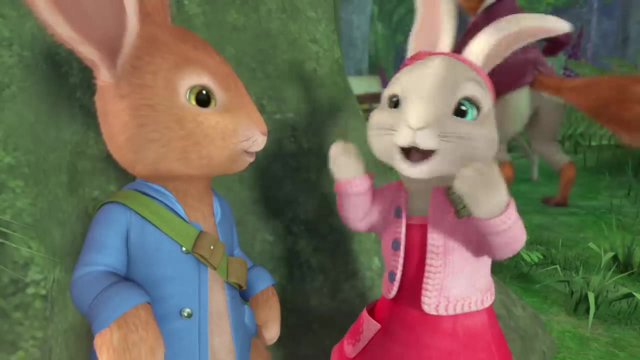 need that fishing rod again, Benjamin. sorry, I left it at the lake. we can make one. I've got some string in a hairpin we could use as a hook, just in case. bucket, just in case I really must be getting back. oh no, I absolutely insist that you. 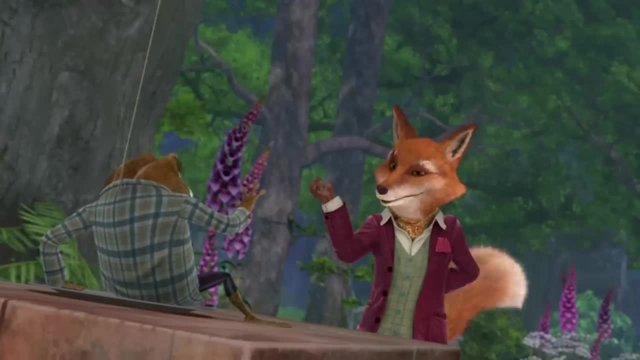 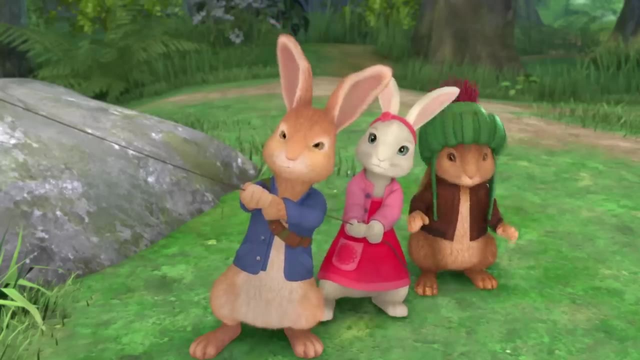 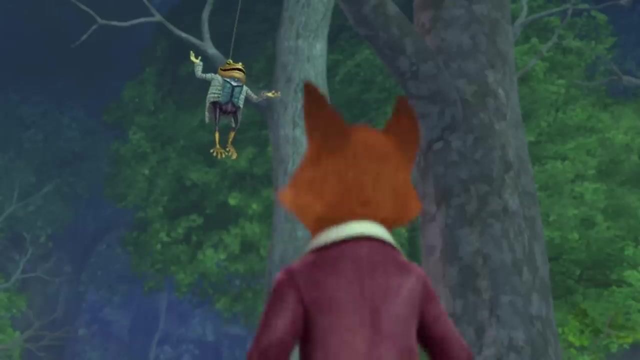 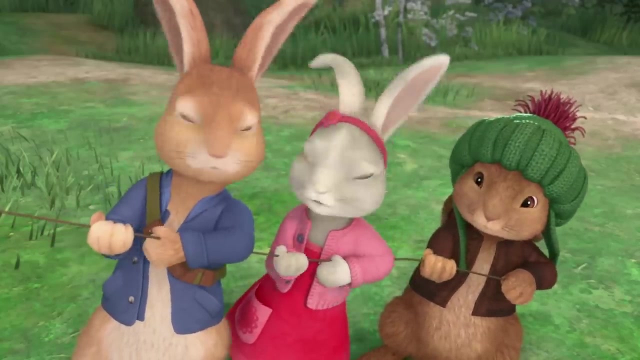 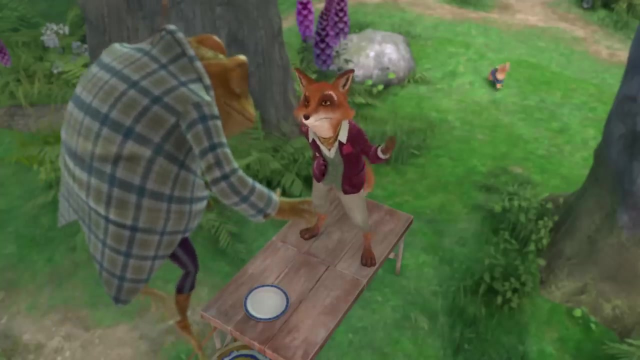 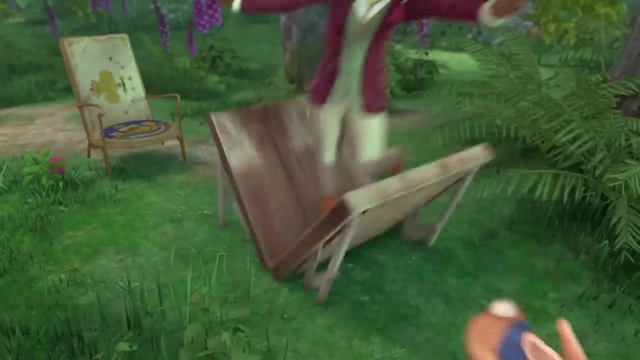 stay for lunch the same without you. I say: where are you going? come down here at once. I think I might hang about up here, if it's all the same. look, aren't supposed to fly and boxes aren't supposed to stand on tables. Oh, Mr Fisher. 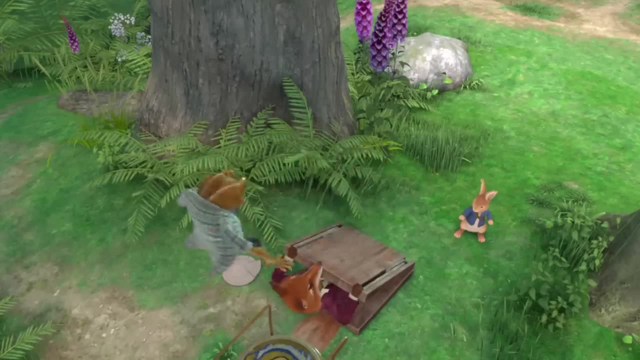 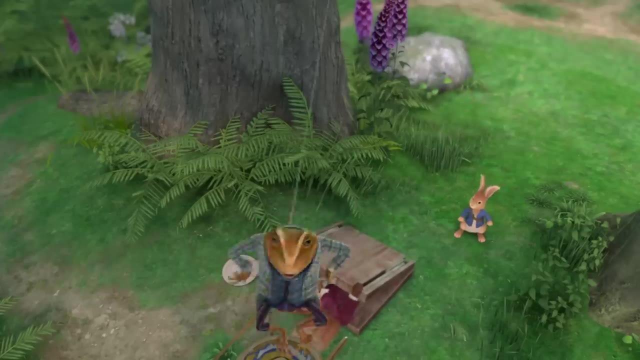 oh, Peter, a rabbit, a rabbit. Not so fast, Peter. I think I've found another exciting musical sound: Creep, La-la-la-la-la-la-la Creep. Be careful, you're swinging too fast, Isn't it marvellous? 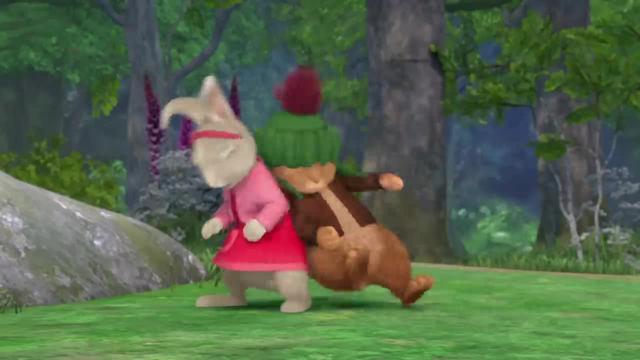 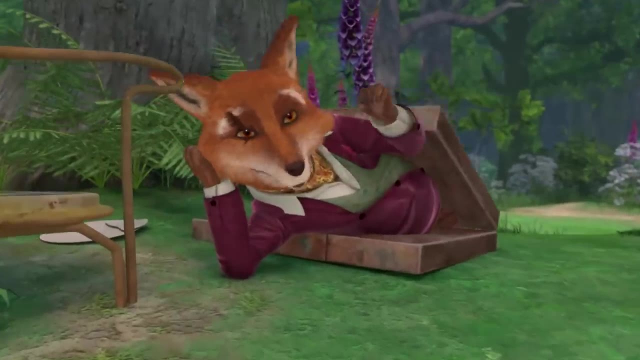 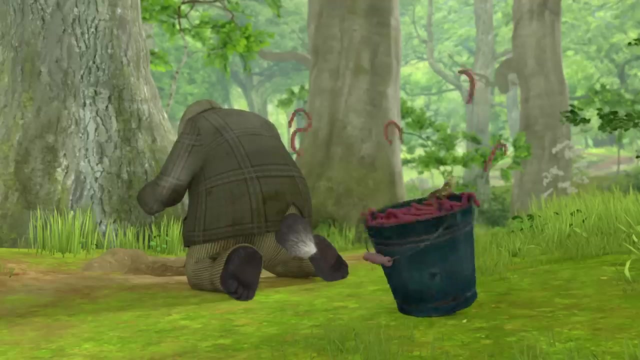 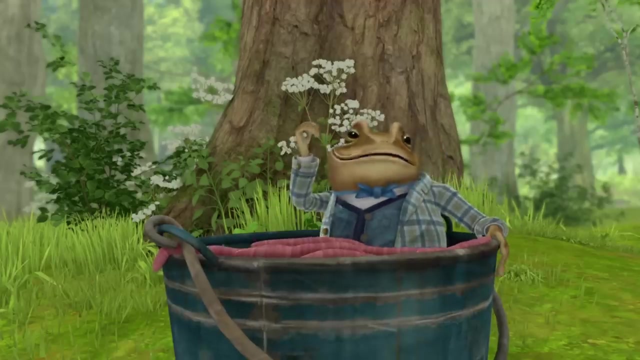 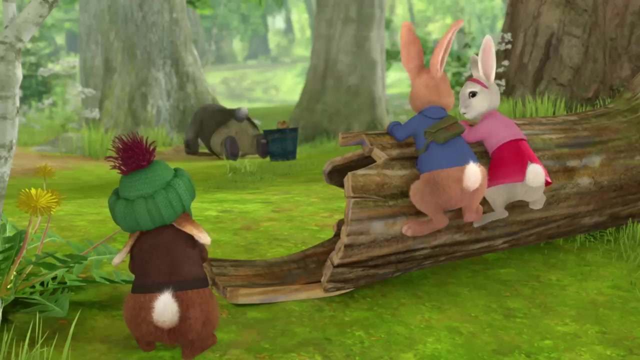 Peter, it's too heavy, He can't hold on. Ah, After him. Why does this always happen to me? Got you What's that noise? Mmm, lovely, If Tommy Brock finds Mr Fisher in his bucket, he'll gobble him up. 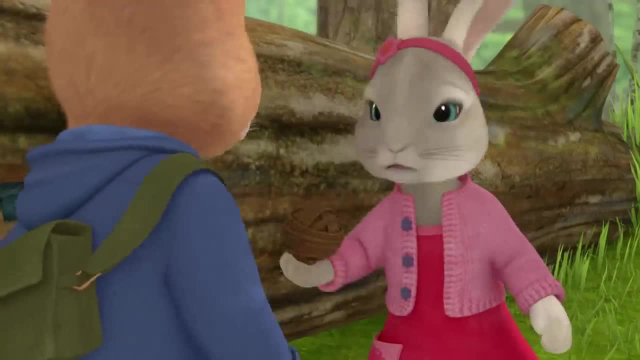 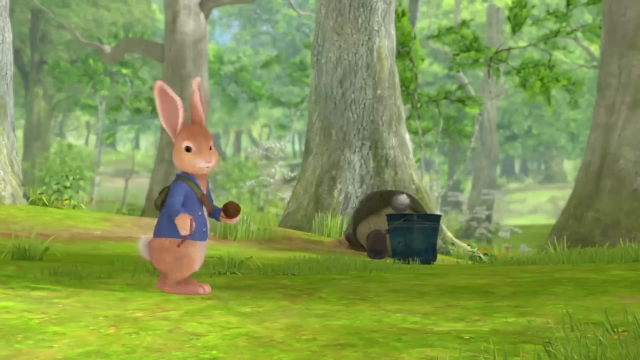 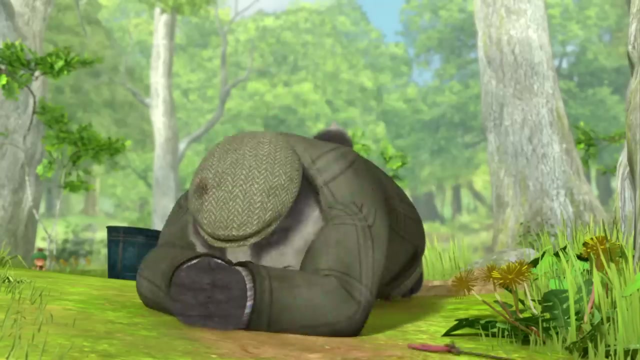 Lily got any more string. Sure, what's the plan When Brock leaves? get Mr Fisher out of the bucket fast. Where are you going? I'm going fishing again, this time for a badger. Mmm, Where'd you go? 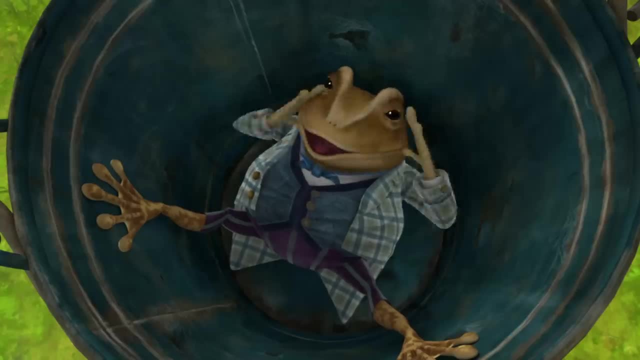 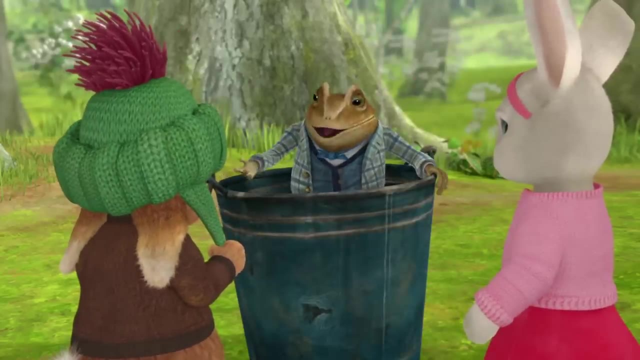